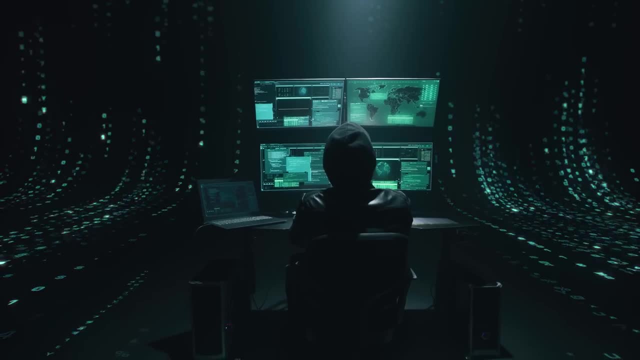 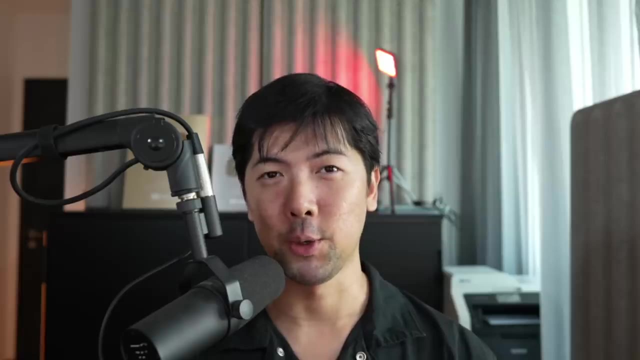 behind a black computer screen with those green color tags, making you look like someone who really knows computers, And if that is what you inspire to be, this is the video that you watch. There are five things that we'll be going through today. The first one is: you need a laptop with an internet. 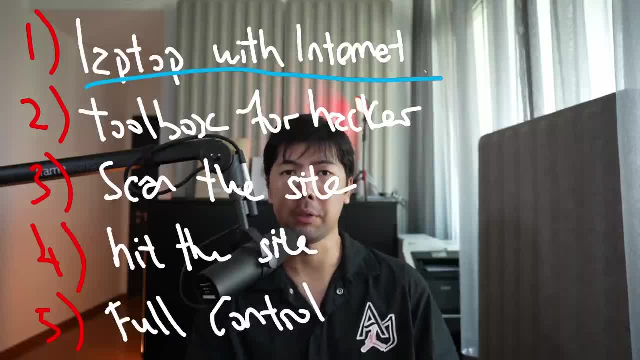 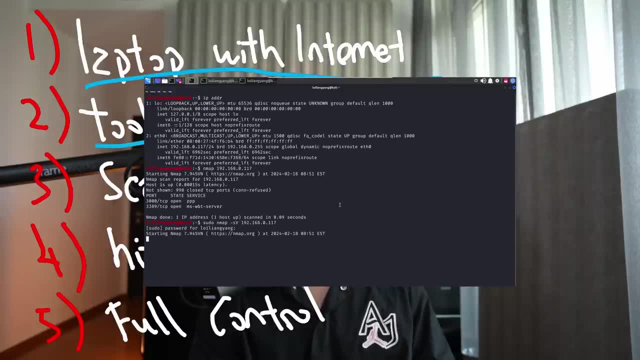 connection. Without internet connection, what are you going to have? Number two: we need a toolbox for hackers, So in this case it could be colonics, which is going to be a penetration testing operating system, Or, at the same time, it could be Parrot OS or even a Windows XP. Number three: we are 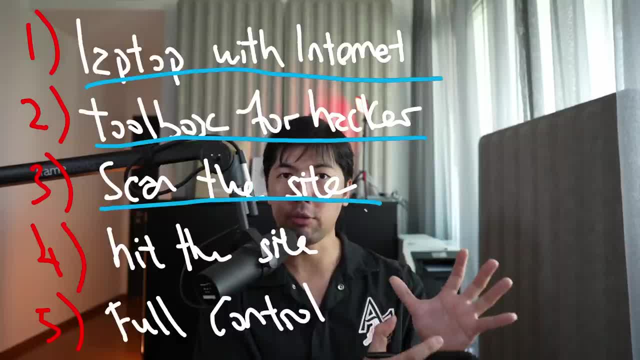 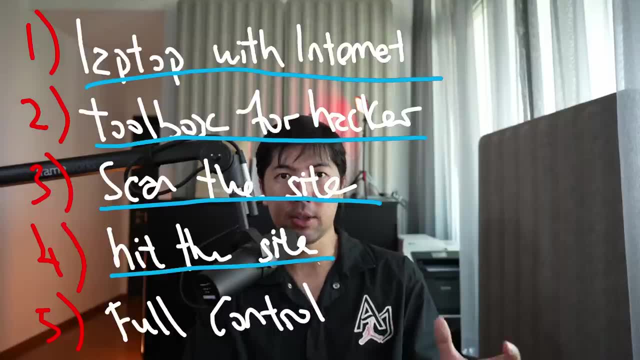 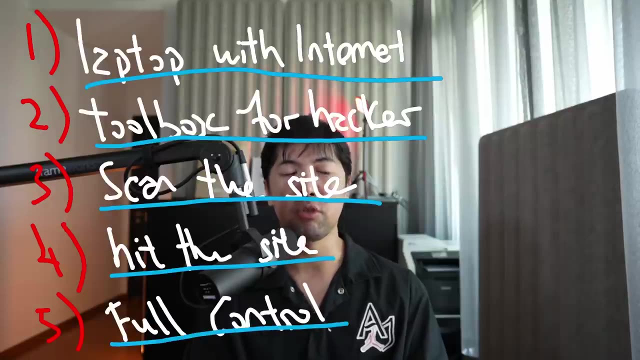 going to scan the target website, looking out for entry points that we can send our code into, so that we are now able to hack into the site, gaining access into usernames, passwords and all the different details And finally, if all goes as planned, we can even have full control of the. 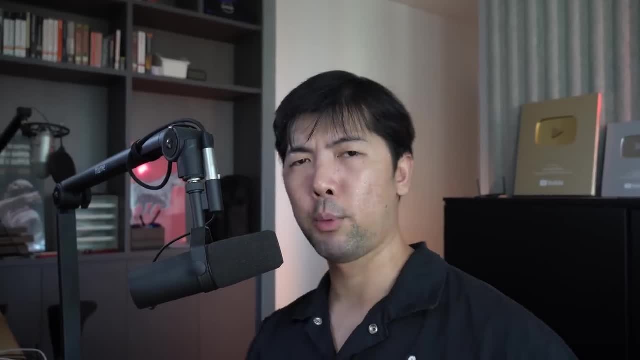 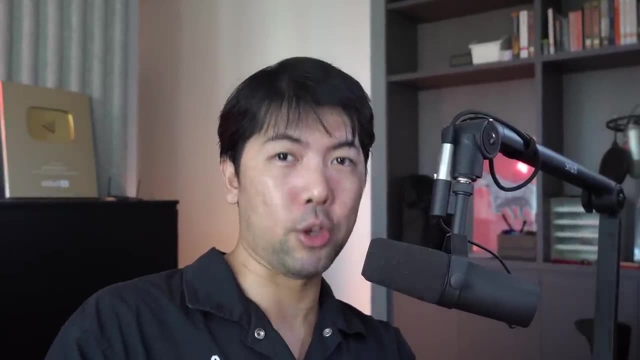 entire system. So let's get started. entire computer, Are you ready? And now, before we go any further, you want to smash the like button and subscribe to the channel so that you get notified whenever I hack you- Sorry, whenever there is a new hacking tutorial. And right in front of us we have Color Linux running This: 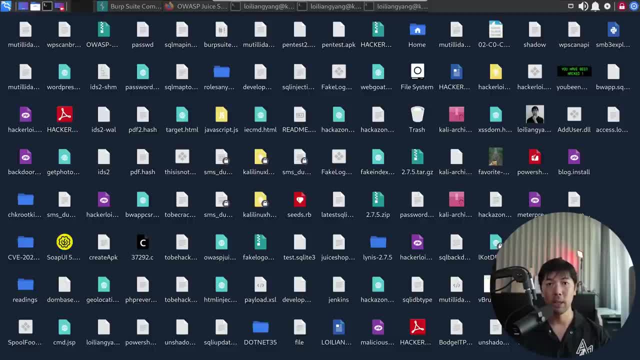 is going to be our article: hacking and penetration testing operating system that we'll be using throughout the whole of tutorial or possibly throughout your whole life, And you can see from the top left corner we have all these different hacking tools, scripts that you can. 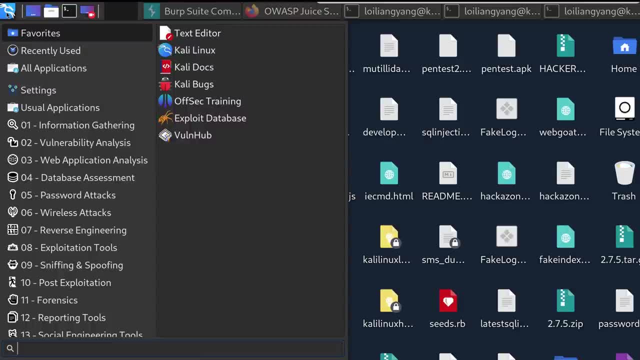 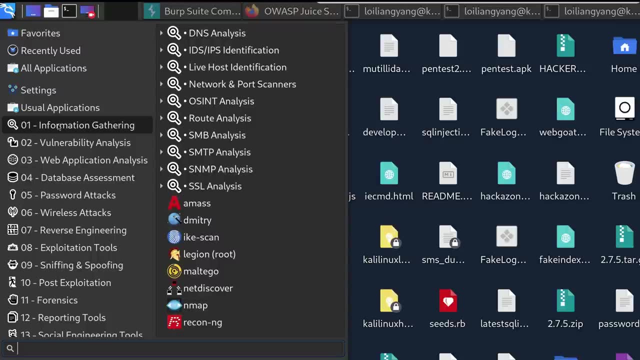 easily use as part of the penetration testing cycle. So, as you can see, here we have things like information gathering to scan the device, scan the website, looking out for and understanding what type of systems languages are the site using so that we can be more targeted, can be more. 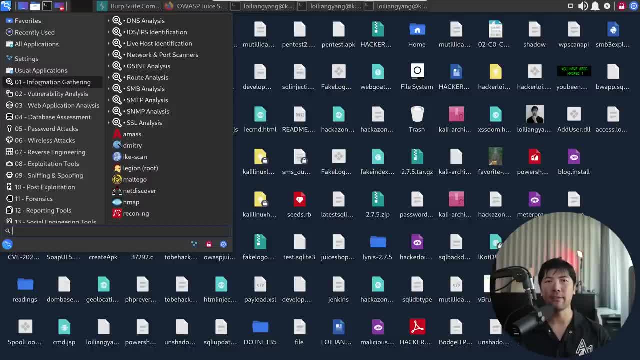 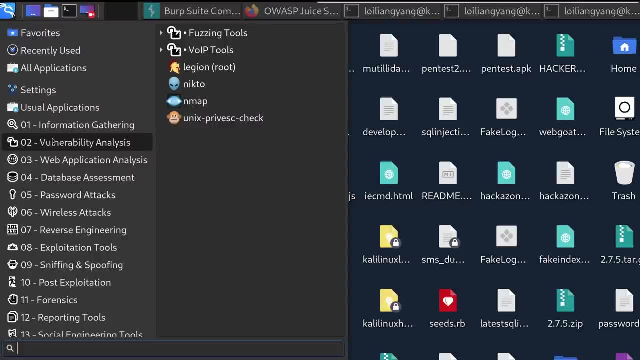 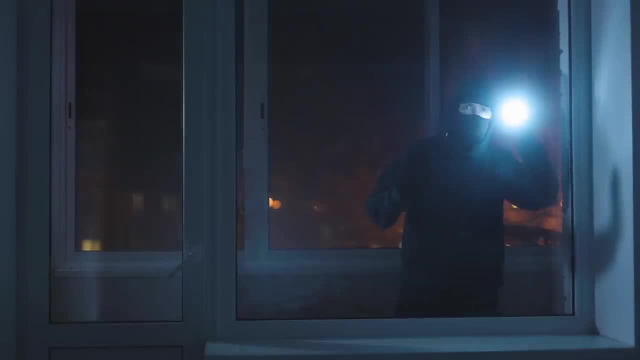 specific when it comes to the hacking part, So you have to do your homework before you start hacking. We have vulnerability. This is the part where we are discovering all these different vulnerabilities and openings. So, just like a house, you are now a burglar. You're going over to a house and seeing where 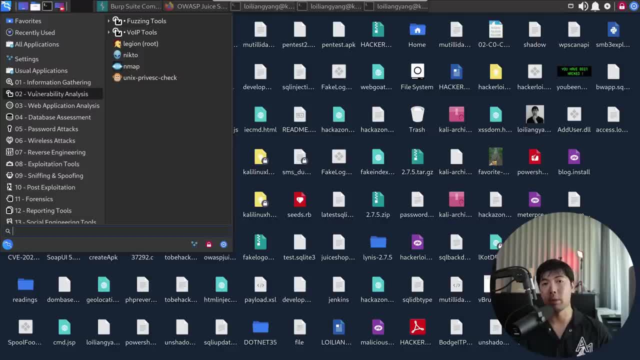 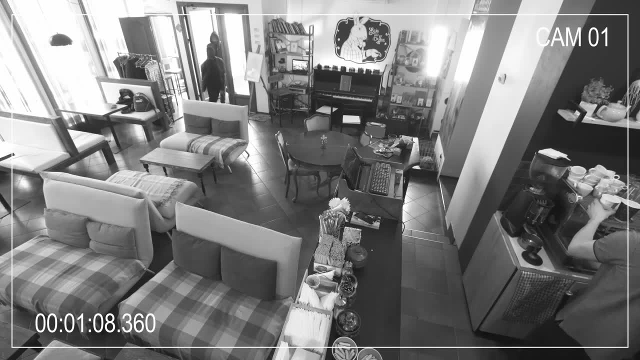 are all the entry points. Is the door locked? Do they have guardrails? Do they have high walls? What kind of security do they have? Do they have CCTV cameras? What kind of CCTV cameras are they using? All of this matters as part of understanding the system, so that we can be more targeted when 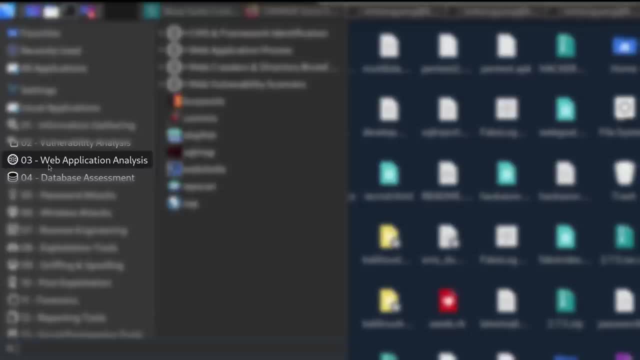 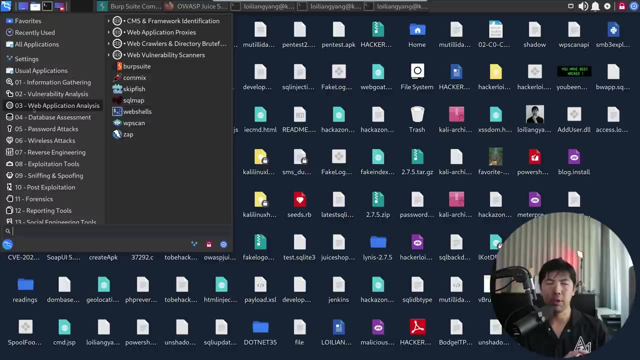 it comes to hacking. Next up, we have web Application analysis, And this is the part where we're targeting a website. We want to understand what is the website running on. What exactly are the different parts of the site that we can target? 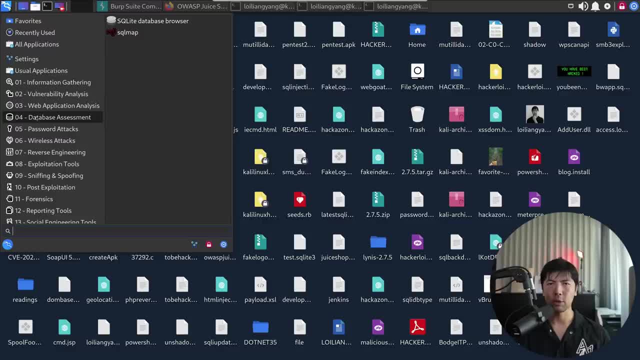 Database assessment. This is the part where the backend system is housing all the system records, like usernames, passwords and all of that, And we are targeting it from here. Password attacks has two types: Online attack, where we're doing things like a brute force login against the system. 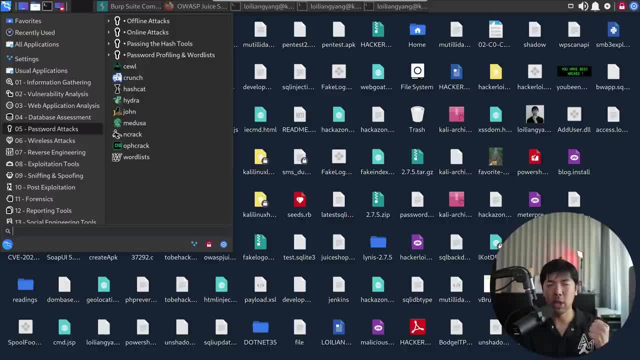 Or number two: we have now extracted all of those Passwords And we want to be able to break those protected passwords. Wireless attacks is where we could be one, targeting all those Wi-Fi within the area, trying to break into those Wi-Fi or creating. 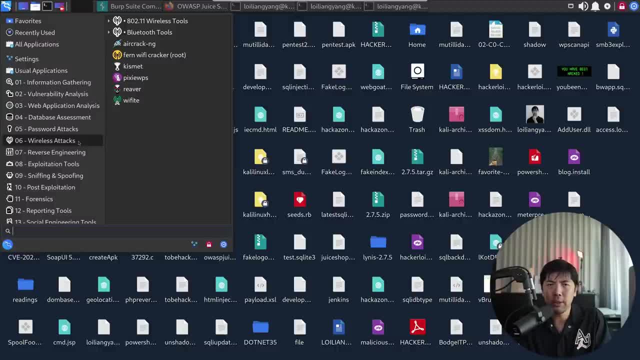 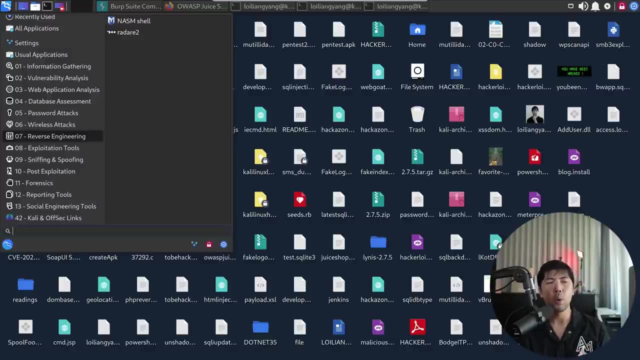 fake Wi-Fi access points so that others log into this fake Wi-Fi access points And we can direct them to some fake social media pages, harvesting their usernames, their passwords, their credentials. Reverse engineering is very exciting. This is the part where we are going to be able to look into an application breaking down the 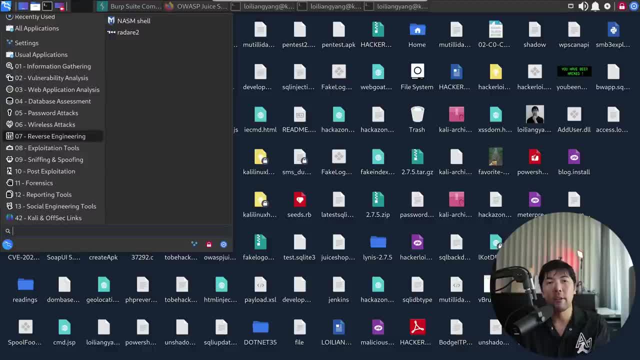 application, seeing specifically where the calls are made and looking for entry points once again so that we can bypass those controls within it. Exploitation tools- the most exciting part of all that you are waiting for, This is where we send malicious code over into the system, giving us 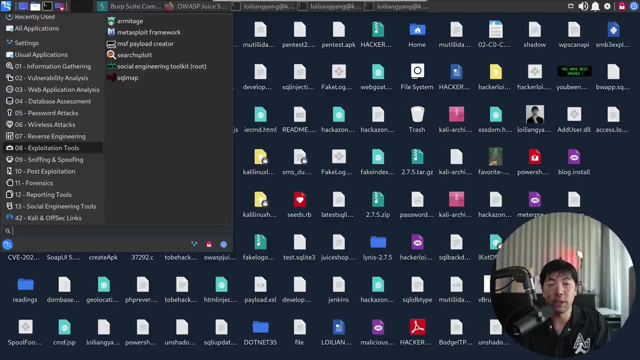 full access into the entire server, into the entire mobile device, into the entire laptop, into many internet connected devices. Are you really aware of all those precise tracking tickets and rapidly Loading and ican dużone application in your mobile or net, Any internet connected devices, Sniffing and spoofing? Do you even know where? 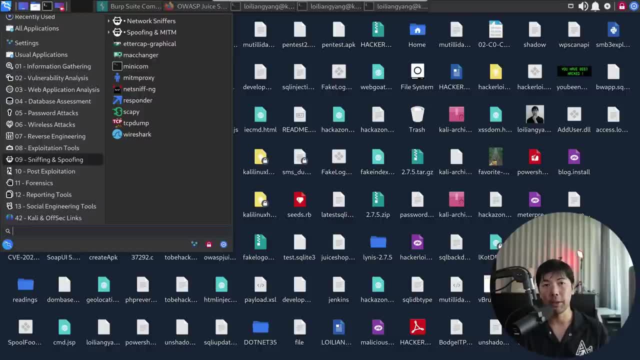 you're maybe at Now, you're actually looking at how the network is connected to Wartime. this is where we help you right away. view this different traffic information to the tools Right here. post exploitation: Now that I have hacked you, what's next? 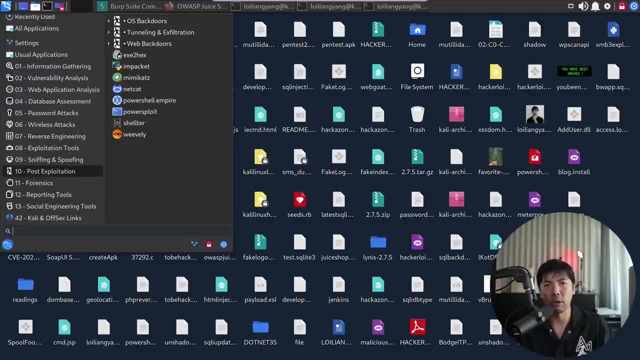 Can I heck Not just your laptop and all of that? Can I hack more of you Forensics? This is where you go to when you know that you've been hacked by me. This is where you try to gather information, artifacts, about what happened in that. 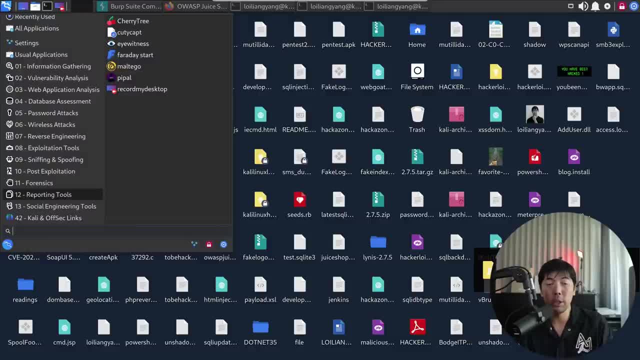 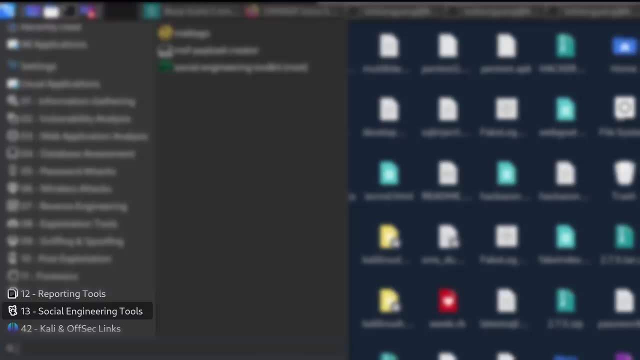 incident Reporting tools: This is where you need to submit a security report to the company that you're doing a penetration testing on And you put your data, put all of those information, evidences, right into a report that is easy to read. Social engineering tools: This is where 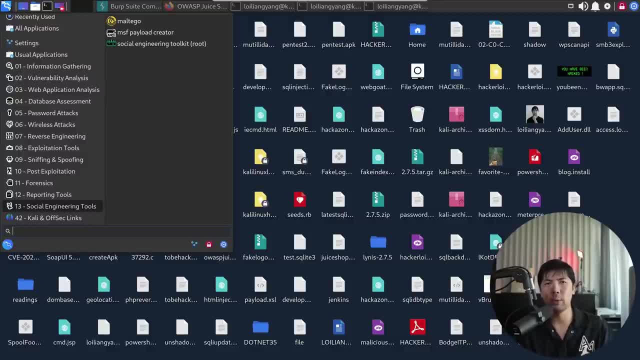 you are being scammed. This is where you go into a site thinking that it is a real login page, but it is not. It is merely harvesting your credentials, Kali and offensive security links. This is the place where you go to, where you want to learn more, where you want to understand more. 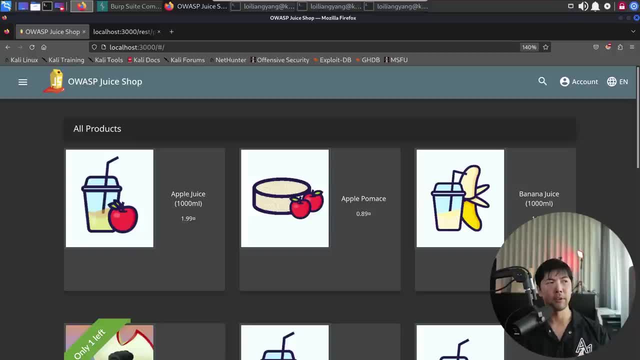 you want to dive deeper into other things. So right in front of us we have OWASP, Which is Open Web Application Security Project, And in this case we have Juice Shop. This is a vulnerable website that you can easily run on your computer so that you can just hack yourself. 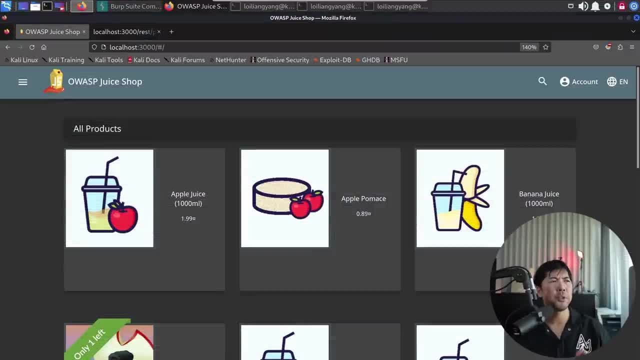 instead of hacking other people's website, The first thing you do is not go ahead and start smashing the hacking button, but instead you want to walk through the site, Gain familiarity with the site, Know exactly what the site is doing. What is it trying to achieve? Where are the entry? 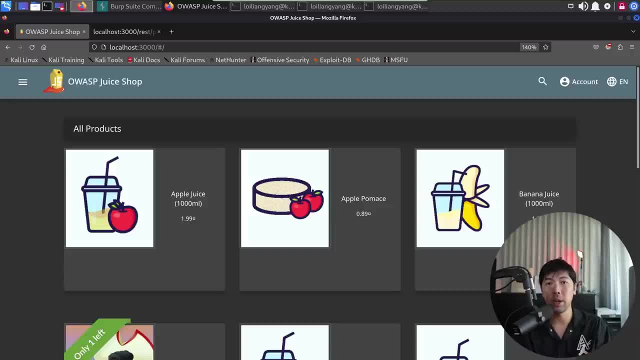 points. How do people log in? What is considered? What are the things that you want to do? What is a normal path for a user? And with that, it allows you to think about all of those other different paths that you can possibly take to gain access into the system, For example, in this case, 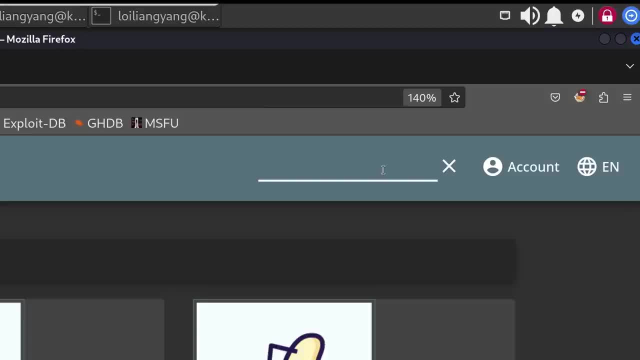 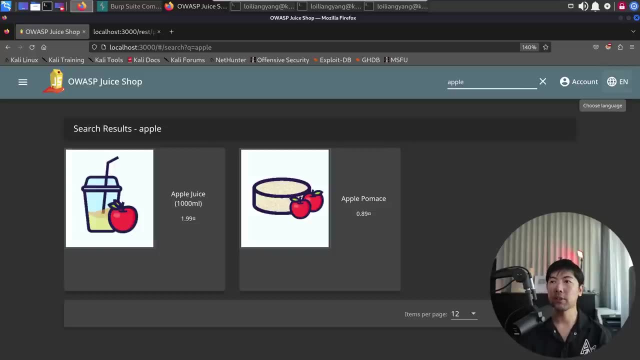 you see a search button right here And I can enter any form of keywords. I enter, say Apple, And I hit enter on that And we can see some results right here. And, of course, there are some slight changes to the website that we are now looking at, which is here: Search Q equal Apple. 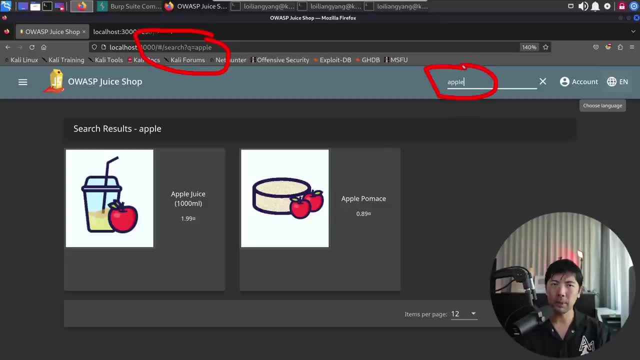 So these are the entry points that we are targeting. So this is the place where we can send malicious code over to the site and think about what can happen when we send those code. And now, if I go ahead and click onto any of the results you can see in this case, 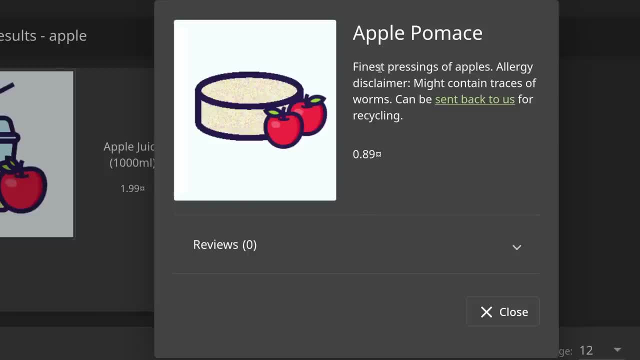 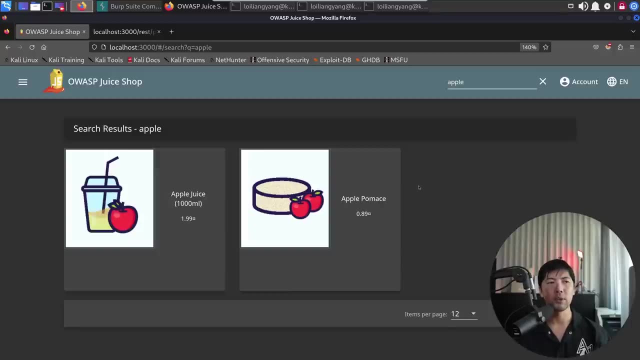 we have Apple per maze, We have reviews, We have the price, We have the description, the product name and so on and so forth. So the first thing that we're going to do right now is to open up the web developer tools. So go over the top right corner, click onto more tools. 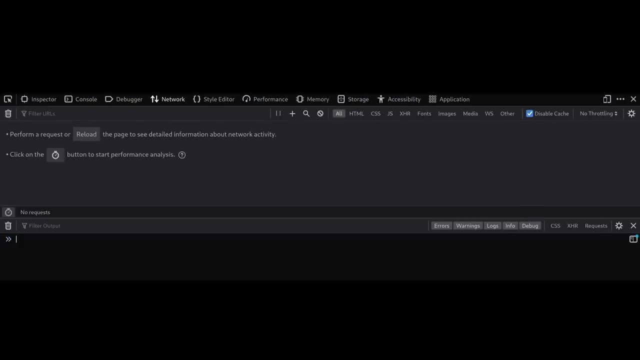 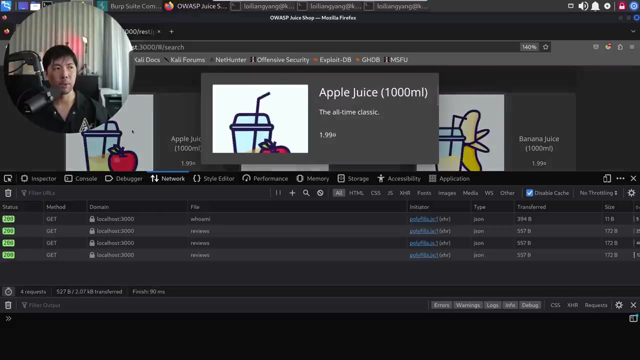 under web developer tools. So from here we can see the network tab. So this will show us how are we interacting with the site. So, for example, in this case, I click onto Apple juice. You can see right here there's a few calls that occurred, For example: who am I Reviews, All right, And 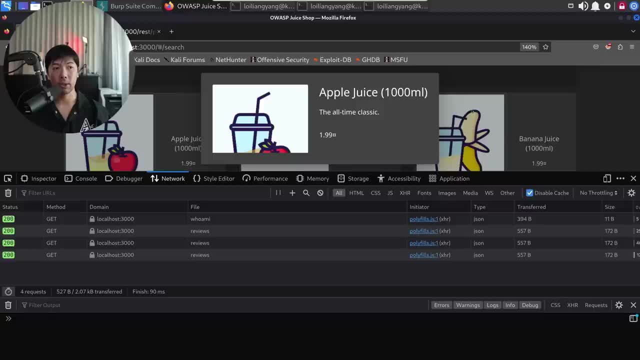 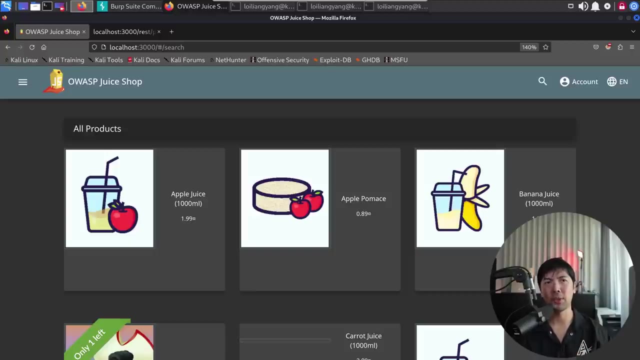 you can see the initiator being polyfusejs. Okay, So we can see. if I click on the banana juice and all these different juices, you'll be able to see how your browser is interacting with the site. Additionally, we can launch specific tools for interception. So in this case, 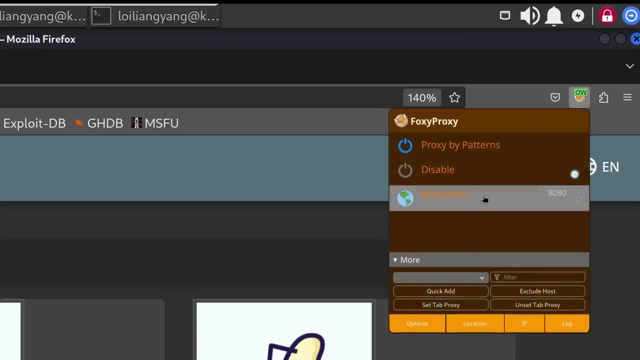 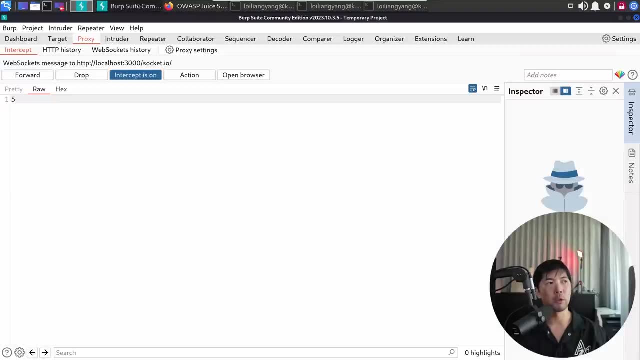 if you go to the top right corner I can click right here We can select under burp suite. So burp suite is going to be a specialized tool for intercepting those requests. So I go over to burp suite right now, which I already have running. I'll go ahead and 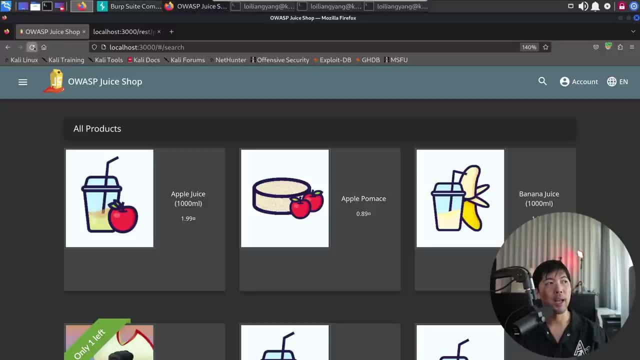 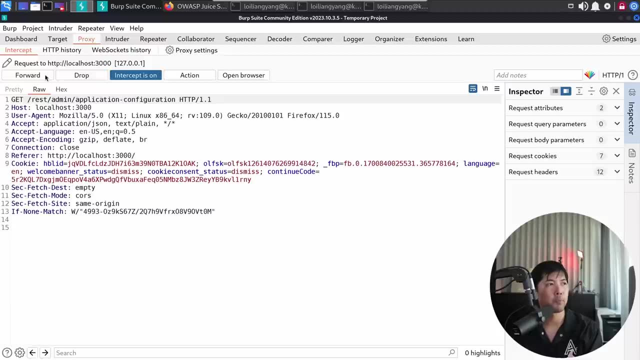 turn on intercept. I go back to juice shop, all to the website. I do a refresh and you can see right here all of the request information and I can click forward on it. And the moment I see something that's interesting, then we can do further analysis on it- I click forward. 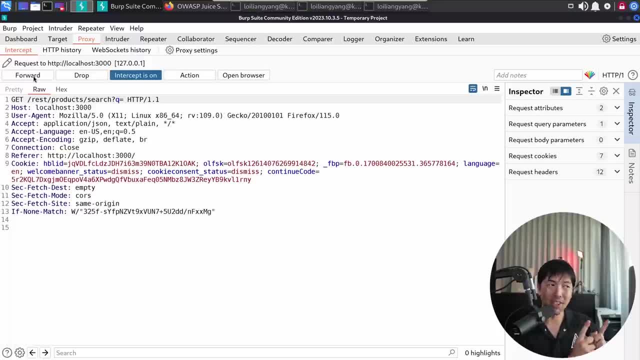 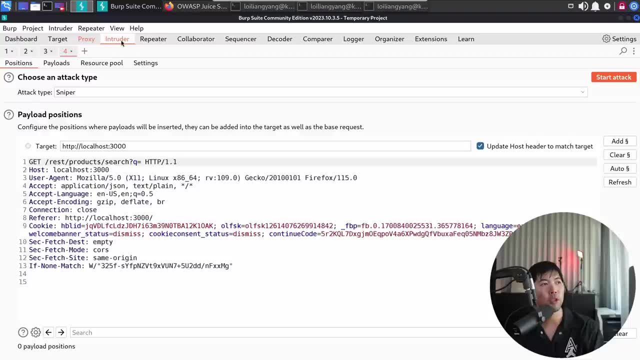 I click forward. So this is the one that we're targeting. This is an entry point. I can do a right click on this and I can send over to say intruder. So once I'm on intruder, this is the part where we could possibly have injection. So in this case you can do a right click, send over to. 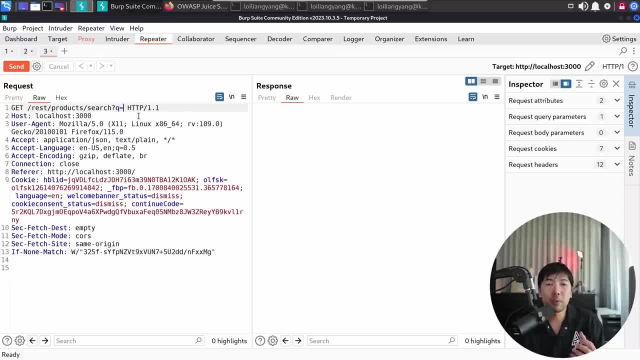 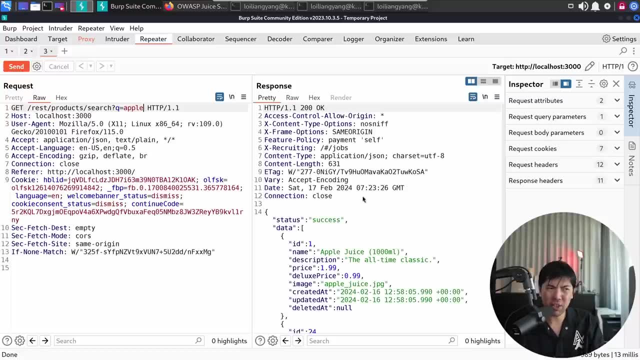 repeater And from repeater I can say: look for more specific things. So let's say, I enter Apple and let's see what is the response. So you can see, here we have HTTP 1.1, 200.. Okay, We have. 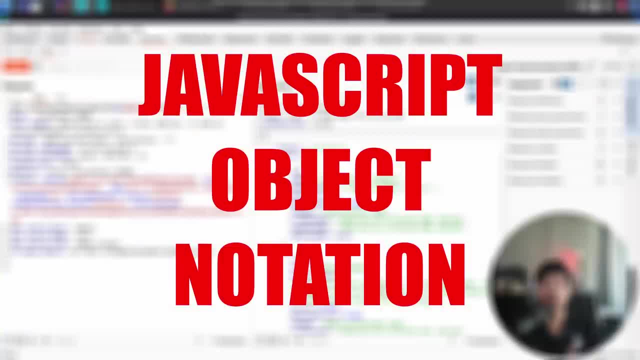 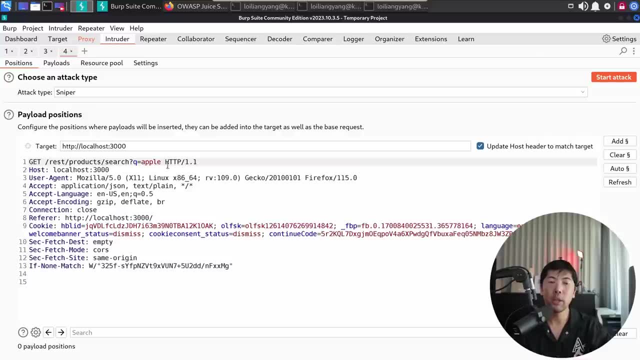 success And the response came back to us in Jason format. Now here's the thing: If I go back over to intruder, what I can do now is can enter, say, Apple, and I'm going to use this to be our marker. 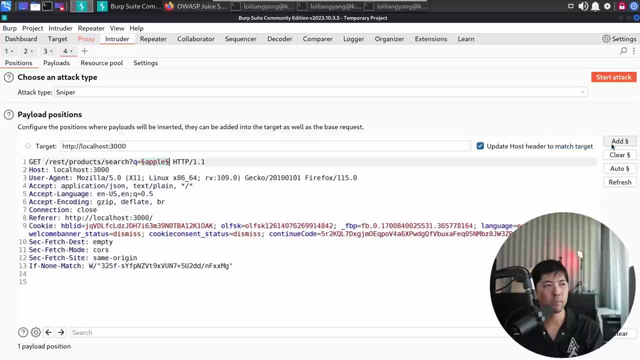 So in this case I click onto add all right payload marker. So this is the place we'll be injecting over into the site. So we'll be sending malicious code and see what happens. So I hit over to the payloads tab, I click onto load, So in this case I can. 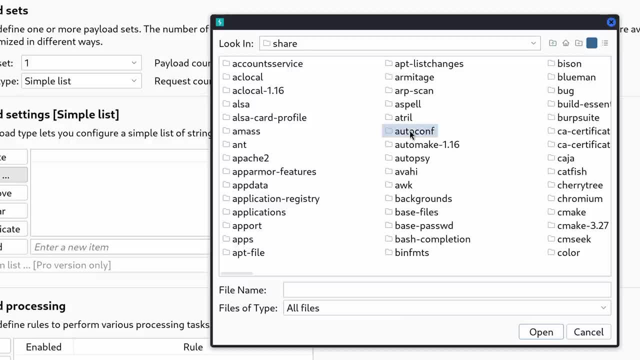 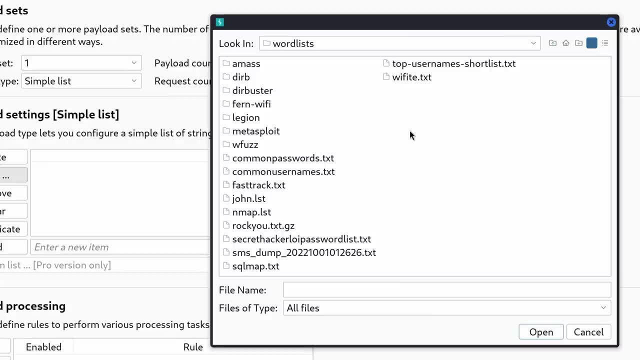 go over into USR share And over here what I can go into is word list and I can look for specific SQL injection payloads, because I want to know what's happening on the back end. I want to see whether we are able to find an entry point that allow us to then dump out everything on the back. 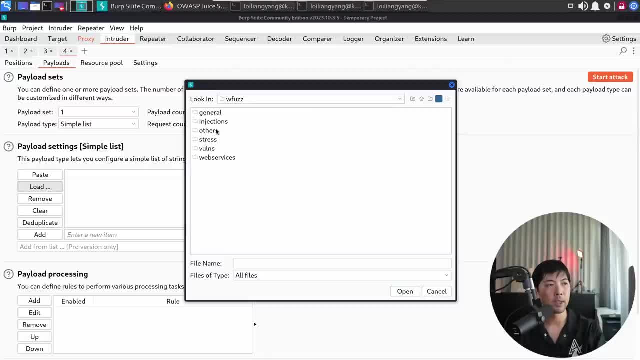 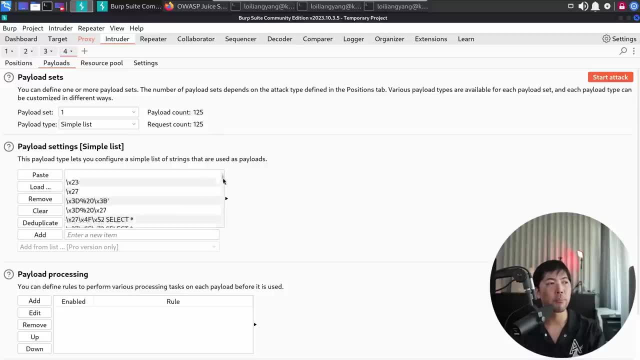 end database So I can go ahead and select onto W fast, Go ahead And click onto injections And in this case sequel dot TXT. So you can see, right here we have a bunch of SQL injection payloads And once you're ready, click on to start attack. 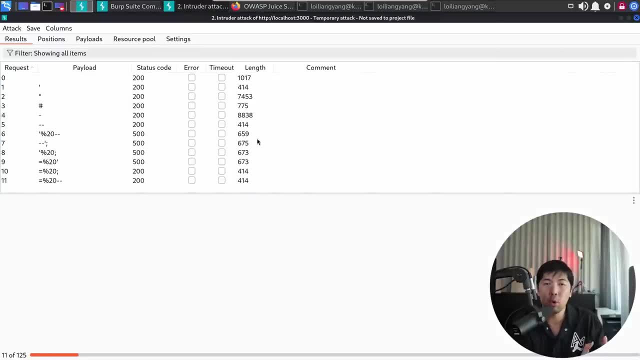 click OK And we're now sending the payload over into the site seeing what kind of response we get as a result of it. So what I'll do now is go over the top left corner, click onto attack. I'll click pause. I want to review the results Now. 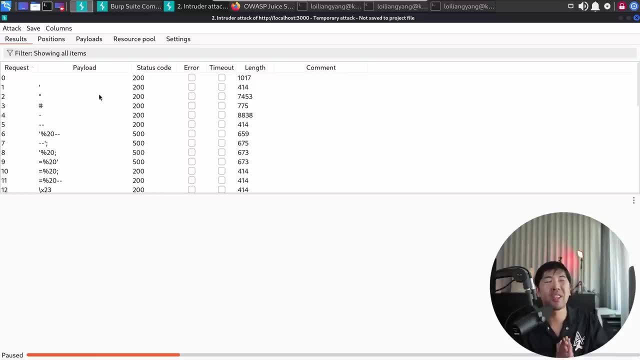 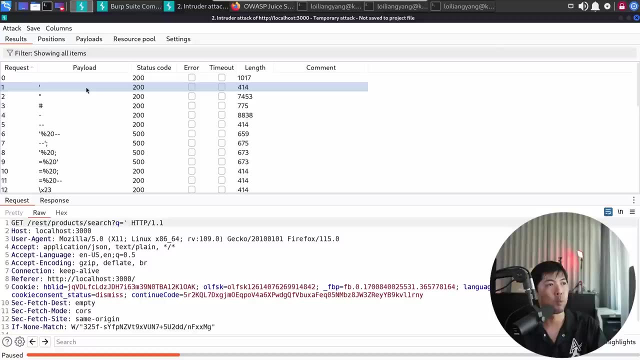 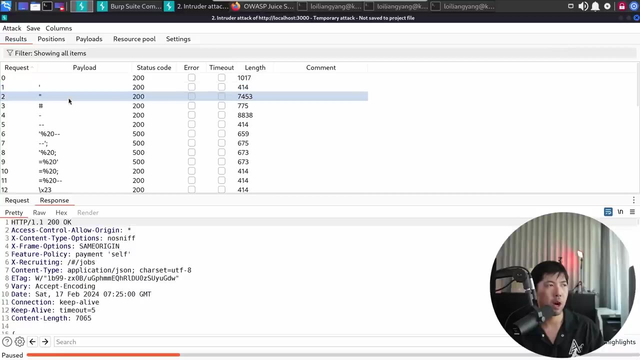 what is going on, which one got us a hit, got us an error message, which we can then continue working on. So I click over into request one and we have the request and the response. So what is the response? success? How about a double quote response? What is the response success? All right, 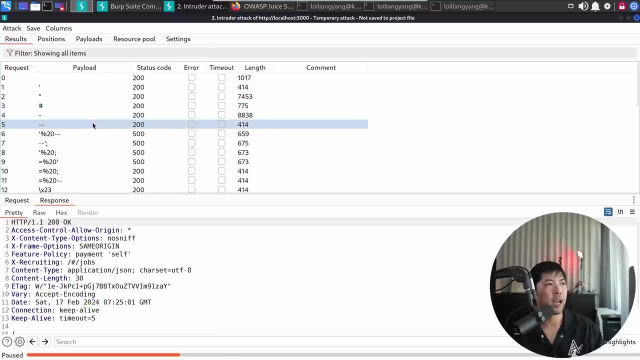 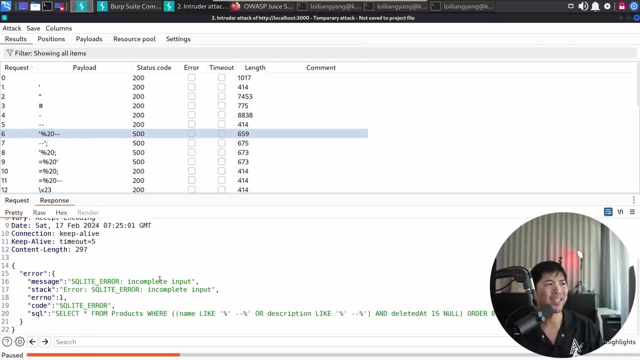 we have hex, we have dash, we have double dash and all these different details right here, And this is the one we are looking for. Number six: we got an error message, And this error message is going to be very important because it displayed to us what kind of structured query 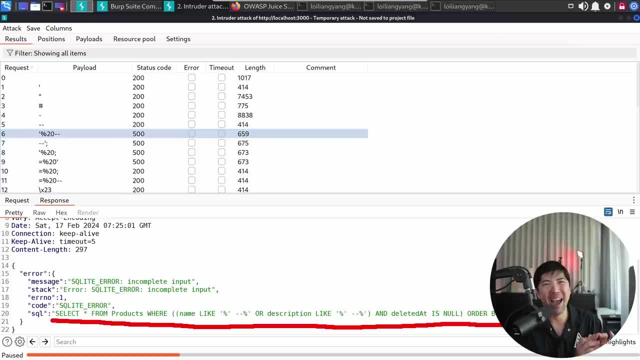 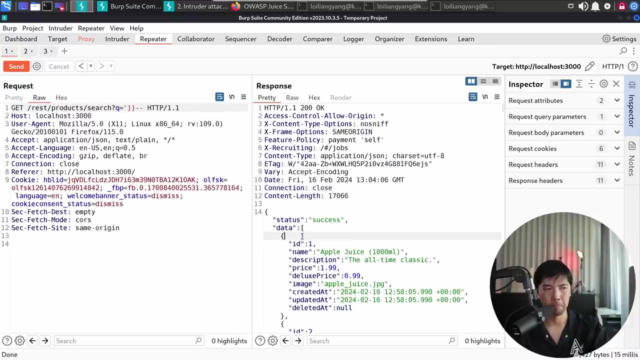 language was being run on the backend, what SQL query is being run, And this allow us to build payloads that will then allow us to dump out every information on the backend system. If you see the request here from the JSON, we have one, two, three, four, five, six, seven, eight, nine. we have nine of 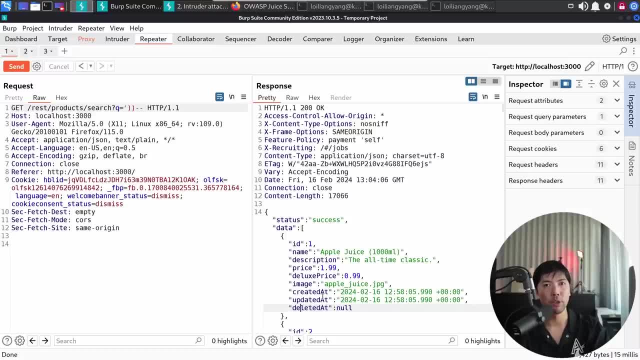 these keys, these key values, And what we want to do now is to think about when we are doing a SQL injection. we want to do a union select, meaning that we are going to pull information out of our tables within the database. The other important point to take note of is we. 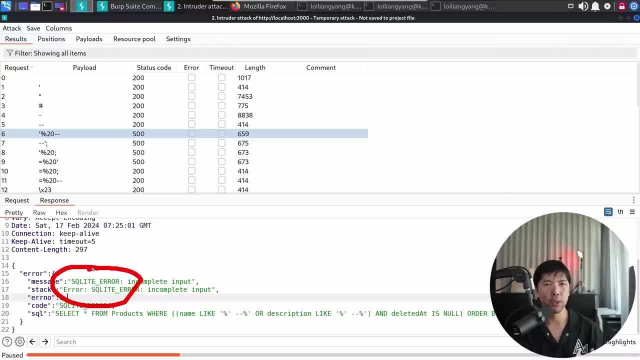 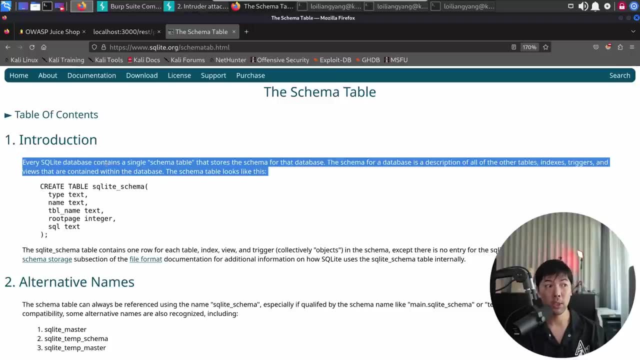 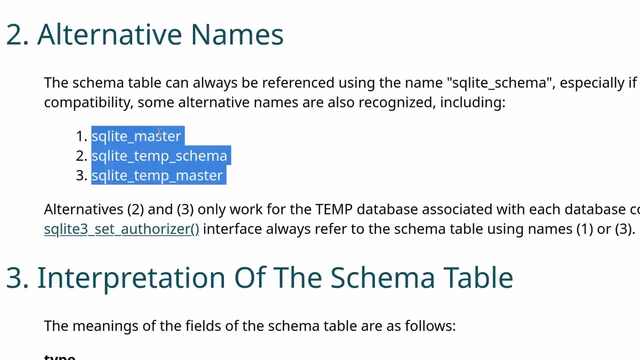 have SQLite error. So it means that the backend database is using SQLite. With that information we can see here, every SQLite database contains a single schema table. So what it means here is there are three names that we can target: SQLite master, SQLite TAM. 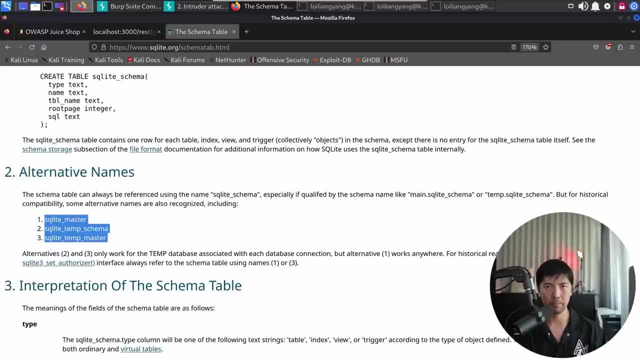 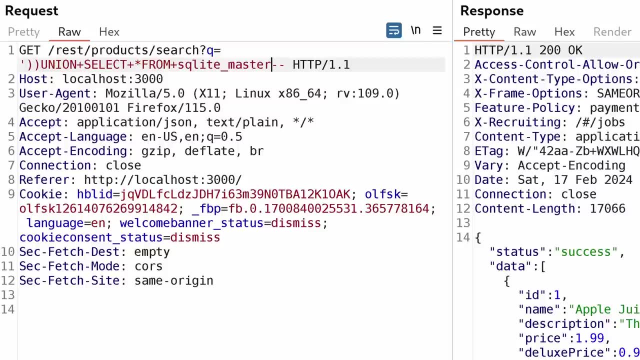 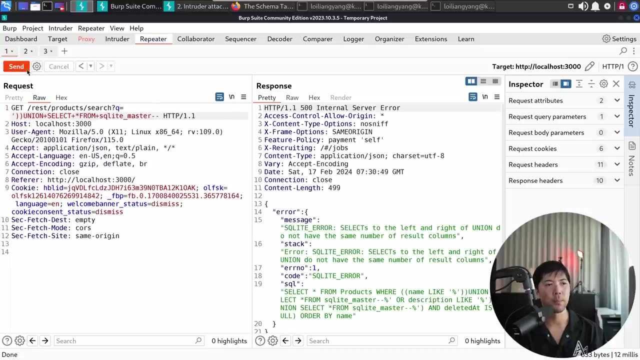 schema: SQLite TAM master. So there is something inside SQLite database that allow us to view those information of tables within the database. So I have a specific payload here that does a union select star from SQLite master. I click send on this. we get the error because remember, we counted, we counted nine columns. So we need 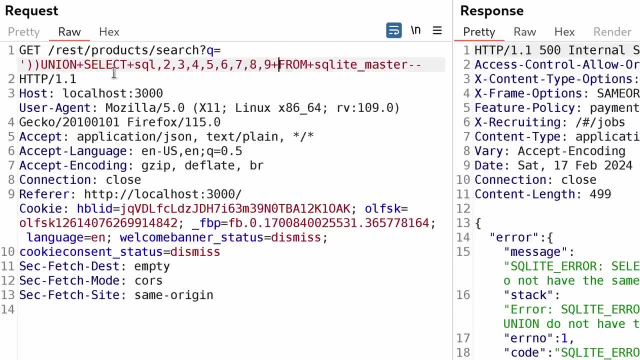 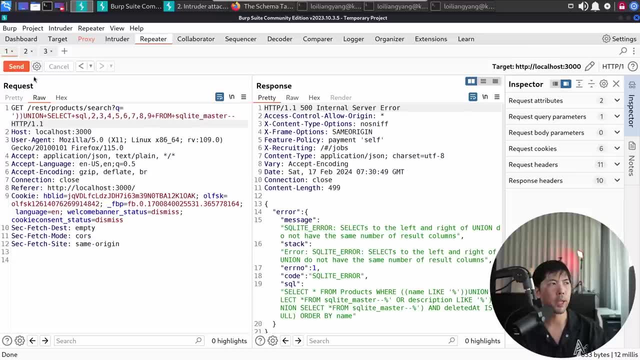 to fill that right in. So I fill it right in now. We have unit select SQL two, three, four, five, six, seven, eight nine from SQLite master. This is a SQL query. I go ahead and click send on that. 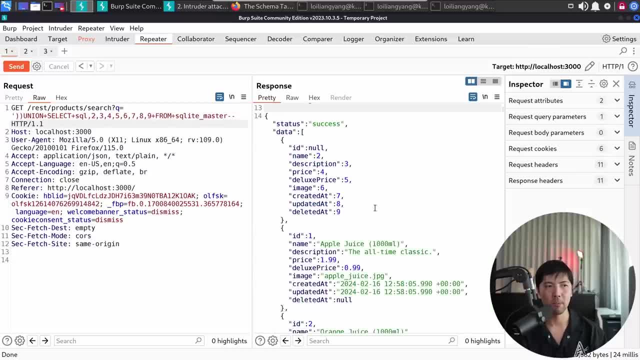 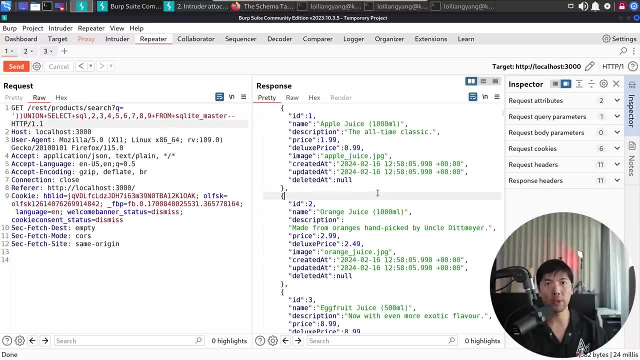 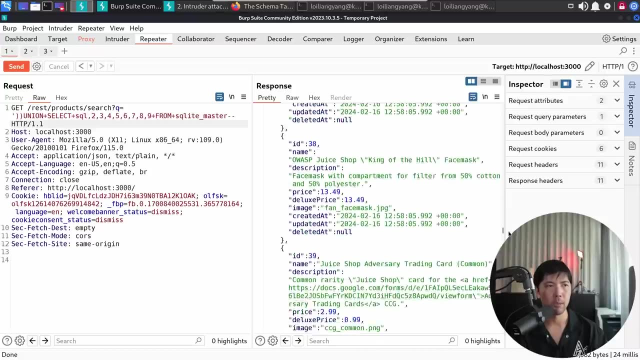 boom done, We have the results. Let's scroll down a little because we have initial results coming in from the table which contains all this different products information. So if I scroll further down, let's go right down to where we can see some interesting information about the database. So if I scroll down further, you can see. 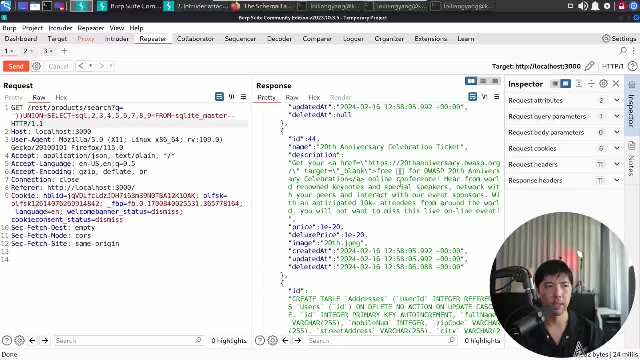 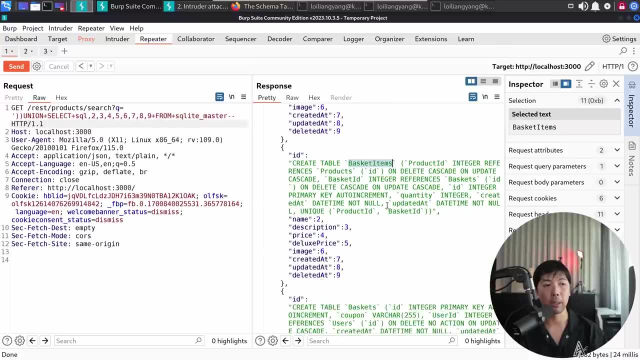 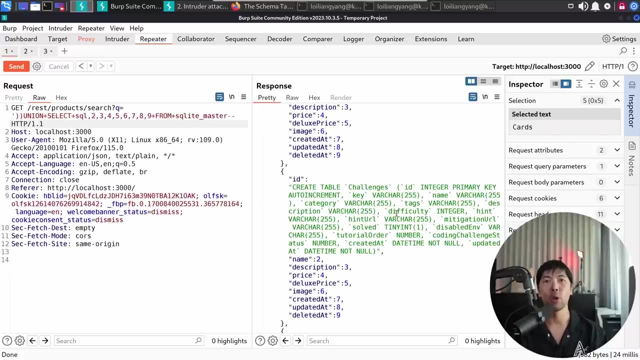 right here. this is the part. This is exactly what we are looking for: Create table addresses, create table basket items, baskets, CAPTCHAs, carts and all these different details. So all these are the different tables within the database. So what we're going to do is we're going to go ahead and create a table. So we're going to go ahead and create a table. So what we're going to do is we're going to go ahead and create a table. So what? 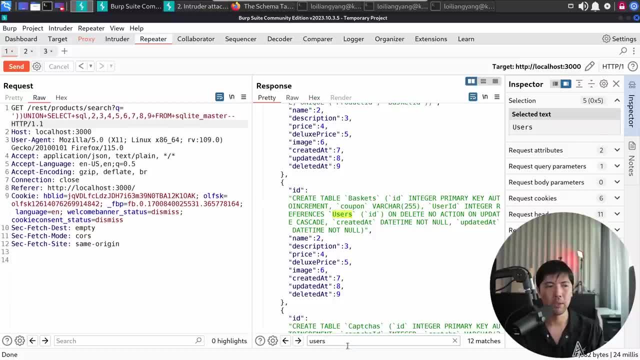 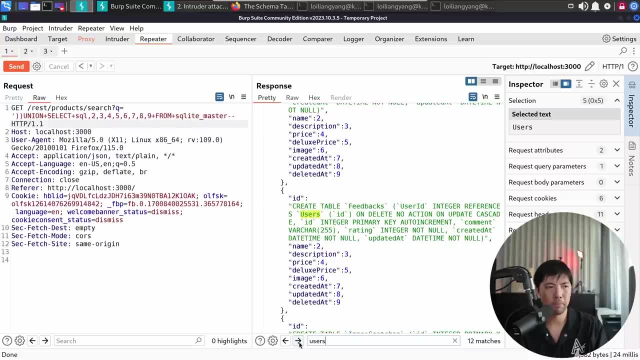 we're going to do is we're going to go ahead and create a table. So what we're really looking for is the users or customers table that can contain passwords, that can contain email addresses, and all this information allow us to start thinking about what. can we target more specifically? Can 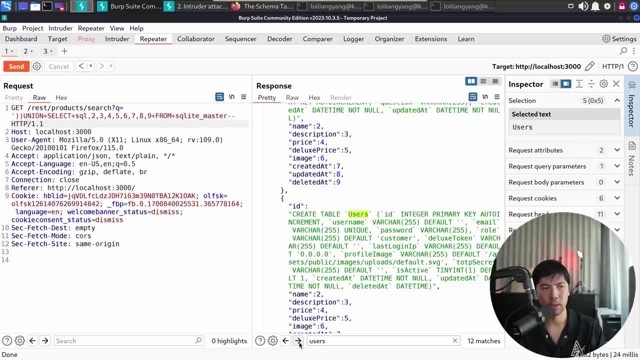 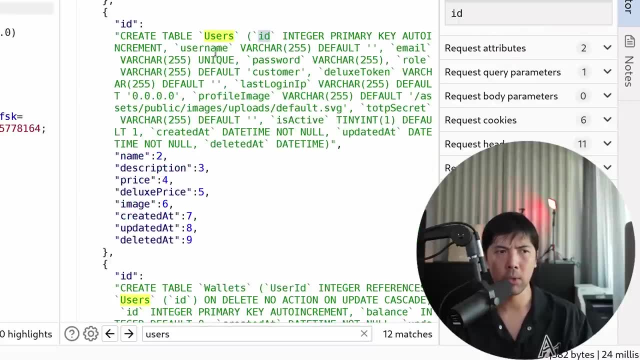 we log in as one of those existing users. So you can see, right here we have the create table users, we have the ID, username, email password and so on and so forth, So we could all this values right here, save them. Now we got a subsequent SQL injection payload In this case. 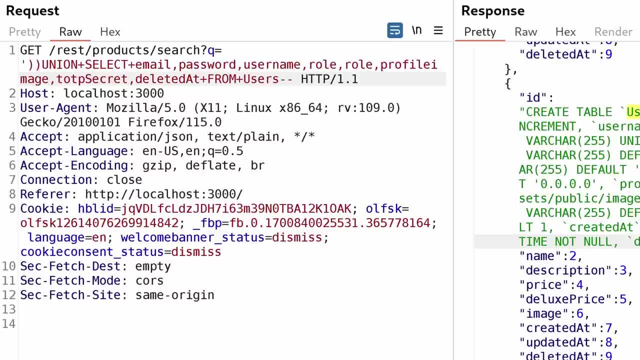 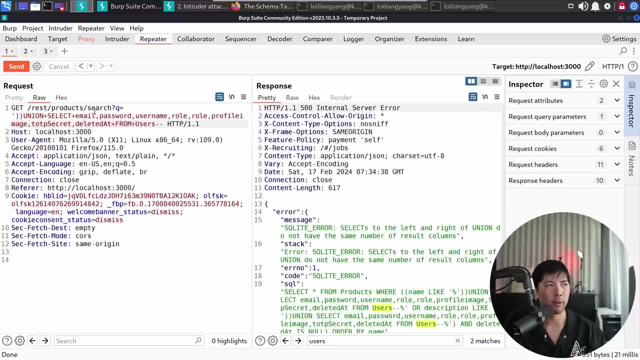 we are going into the users table, we're trying to figure out what are the passwords And I can go ahead and click send on this. Okay, we got some SQL error, So let's go ahead and investigate on that. union select email password, username role- all we got two roles, So perhaps we're going to 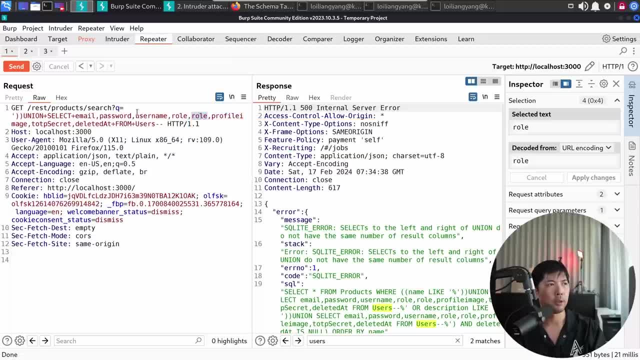 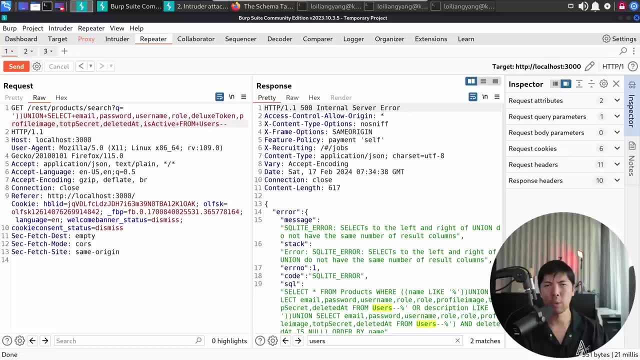 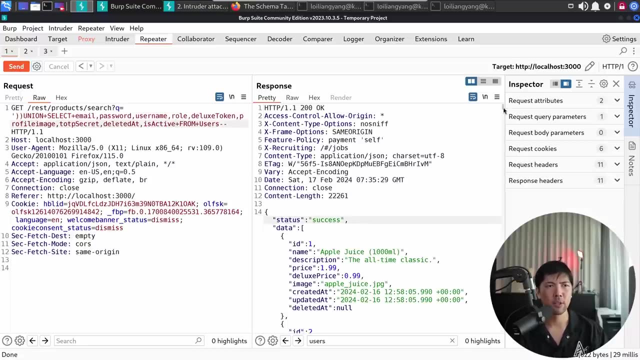 change this up a little bit, Would that be correct? So we got one, two, three, four, five, six, seven, eight, eight. So we need one more column. Okay, good news, Welcome back. So go ahead and click send on this. Boom Done. Let's scroll down, moving away from the initial results. 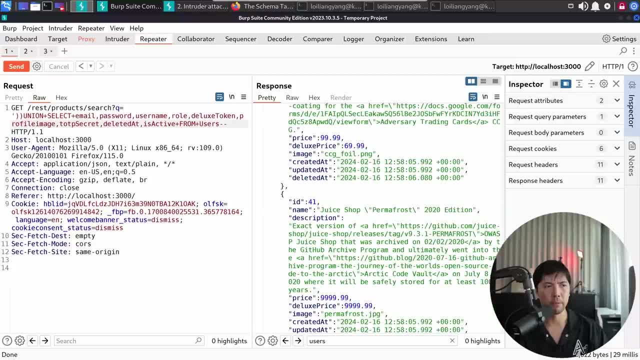 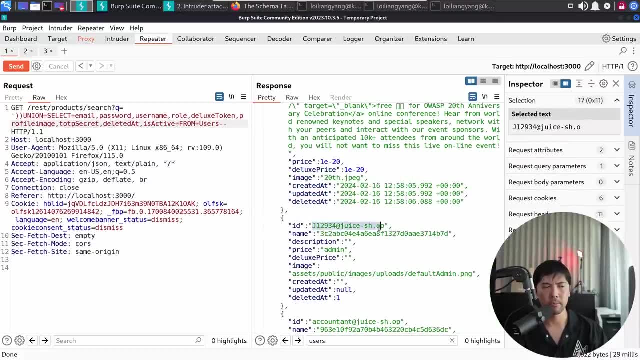 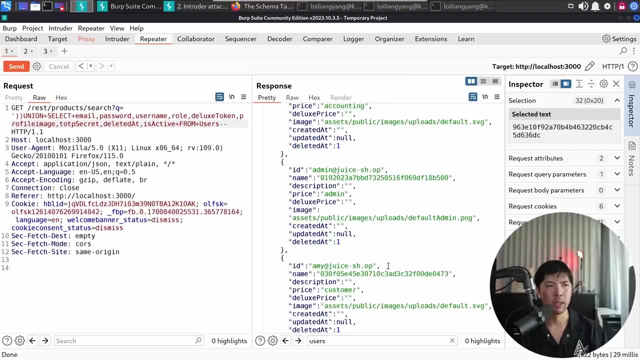 of all those products And if we scroll down further, we can see right here. Let's see, let's see what we get right here. This is it. This is first the email password, another email, another password, so many of them, And we can easily log in right now. 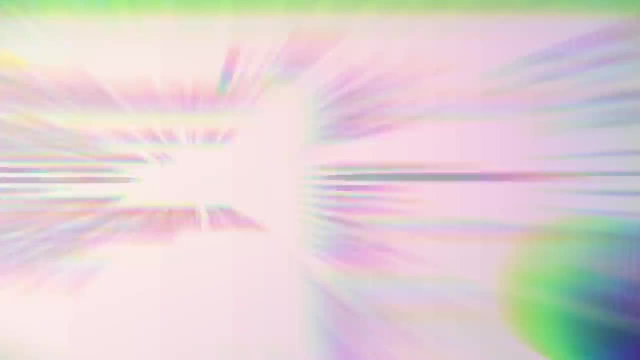 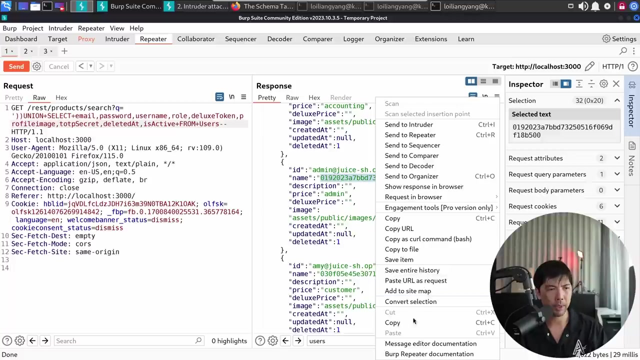 Now, quite clearly, the password is some kind of protected password. It went through some kind of mathematical processing. So what we can do here is we can use some kind of identifier So I can copy the value, I can go over into terminal and I can say: enter the following of: 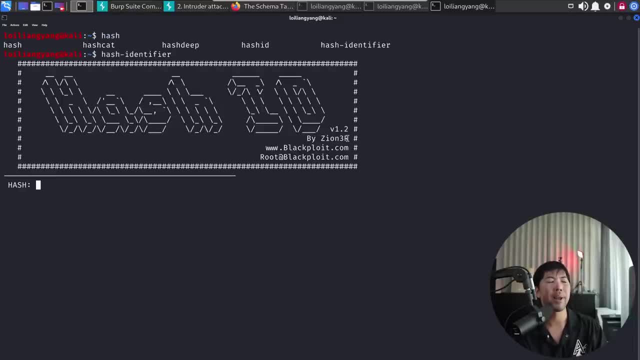 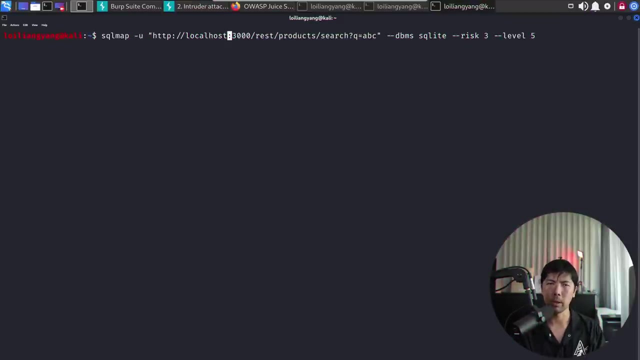 hash identifier. hit enter on that and paste the value right here. Hit enter on that and let's see what it tells us. It states the following possible hashes: mv5.. Now I know we have done all of this manually and there are tools out there that can speed up that. 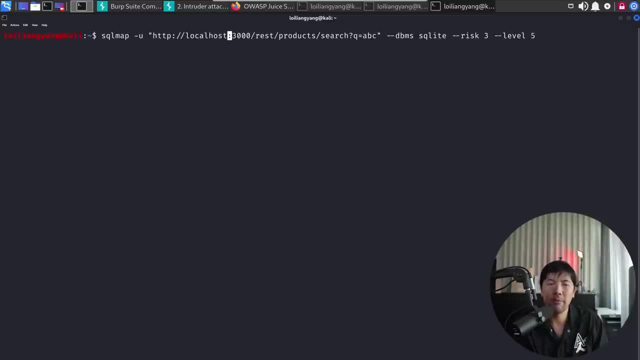 process, And it's important that we learn how to do it manually before you use those scripts or tools, because you don't want to become a script kitty. So what you can do now is go ahead and enter the following of SQL map targeting the URI, And then from here: 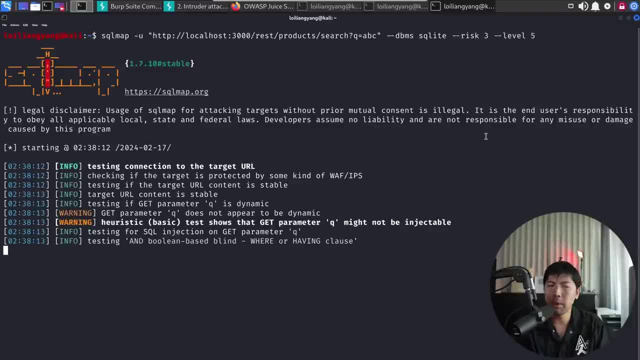 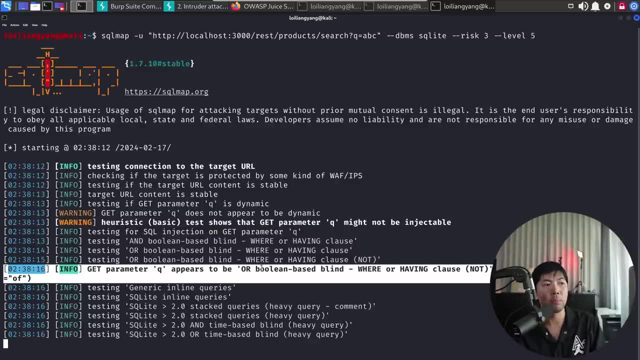 we can go ahead and hit enter on that And let's see what we get. It states the following: get parameters queue might not be injectable. Get parameter queue appears to be for boolean were injectable. Okay, So we are doing the testing right now. We're seeing what we get. 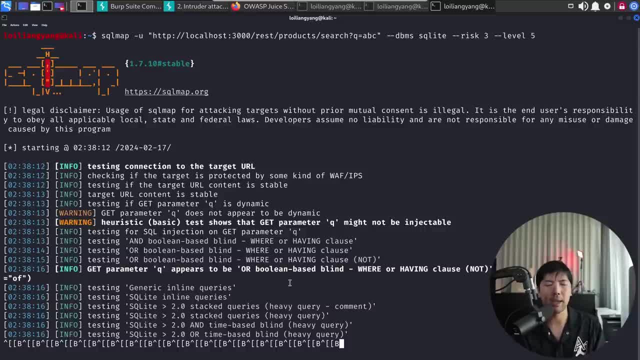 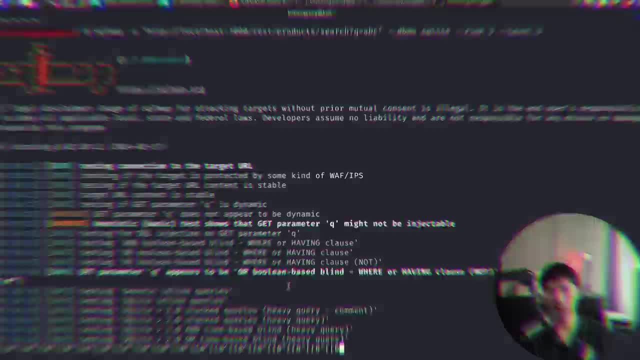 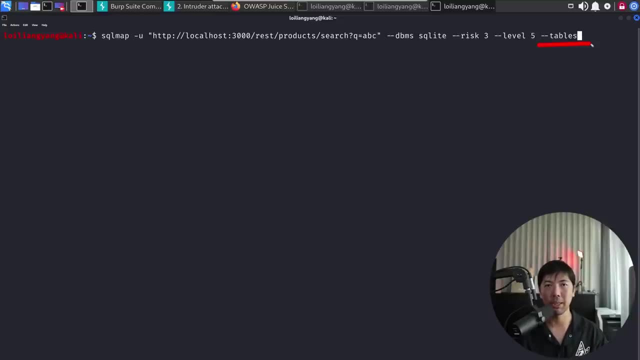 as a result of it. So the tool automatically injects those payload for us and then tell us whether we are able to gain access to the backend database. And I've added one more option here: dash, dash tables to dump out all the tables within the backend database Run. 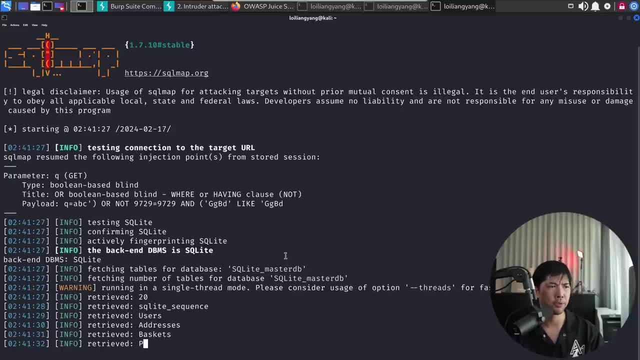 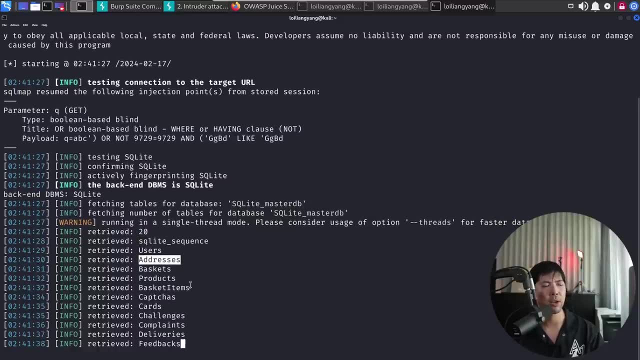 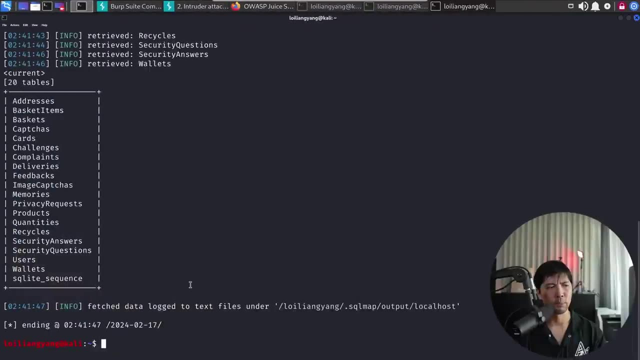 Let's see what's happening right now. You can see fetching tables for database SQL like master, DB SQL like sequence users addresses baskets, products, basket items and so on. This is the same result that we got earlier when we're doing the manual injection. Isn't this beautiful? 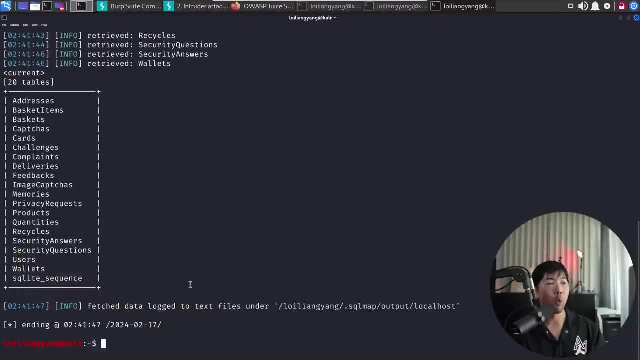 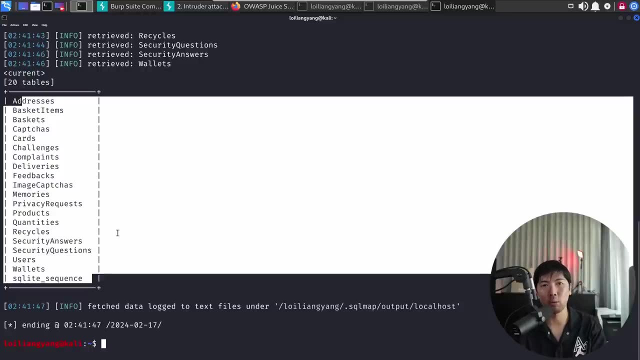 Completely automated And we have identified 20 tables, So you can see all of them right here and we can target them more specifically using this automated tool. Now, this is the exciting part that you're waiting for. We've run a following SQL map: 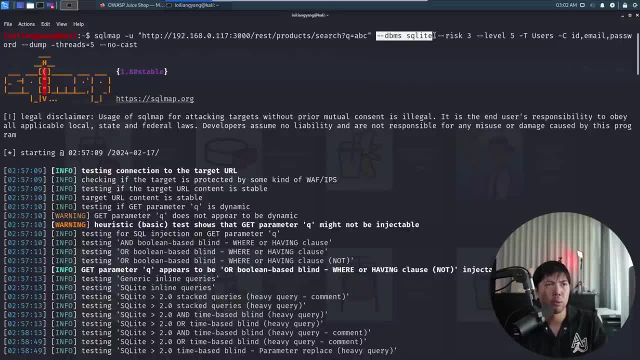 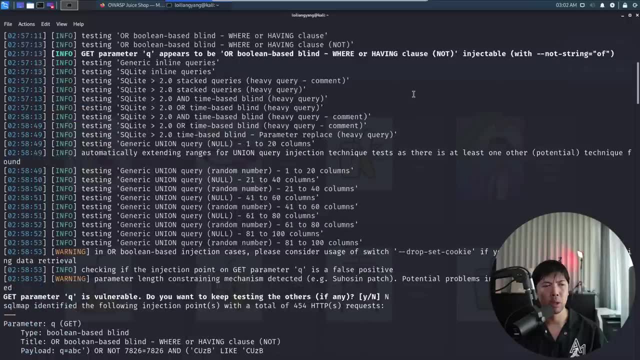 and I'm using it on a computer. Now we're targeting SQL live with risk level. We're targeting columns of ID, email and password, even dumping up all this information. And right here we managed to pull up all those information, similar to the manual injection that we did. 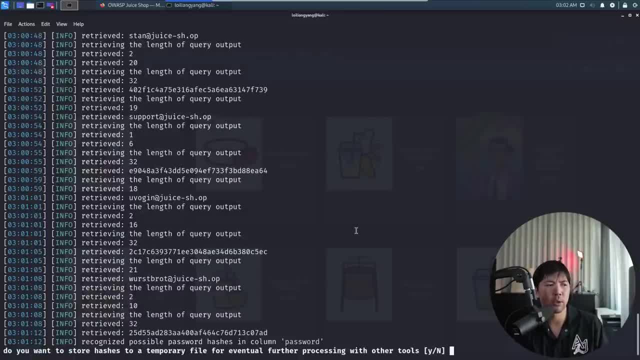 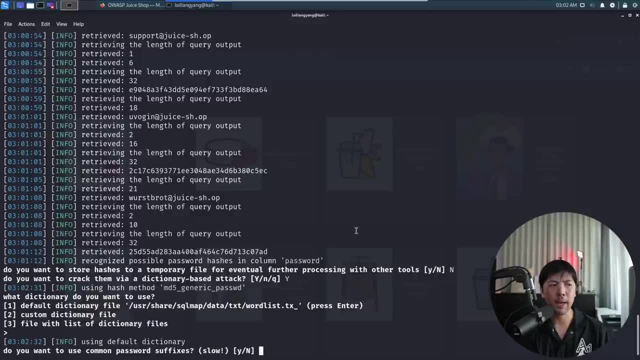 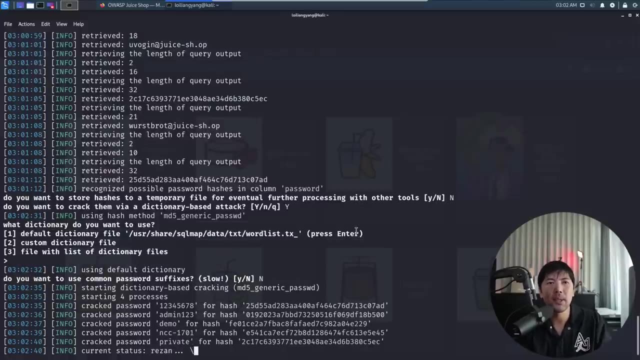 earlier, So right now. it states the following: Do you want to For hashes, do a temporary file enter? no, for that, Crack them via dictionary base: attack: Yes, Hit enter on that. No common password suffixes. Now we are cracking the password. live and let's. 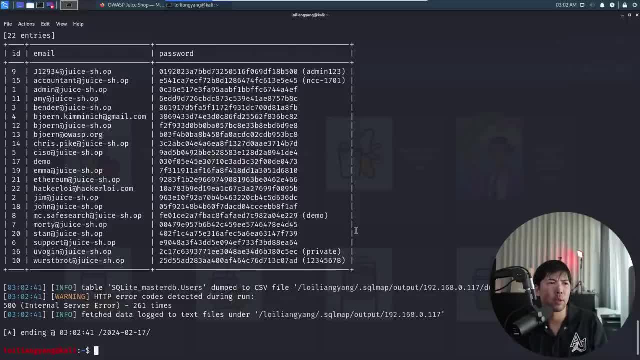 see what we get. Do we get all of the passwords for all of the users? So this is something that we can do, but of course there are also situations. There are also situations where it is not properly sorted. So if we look and compare, 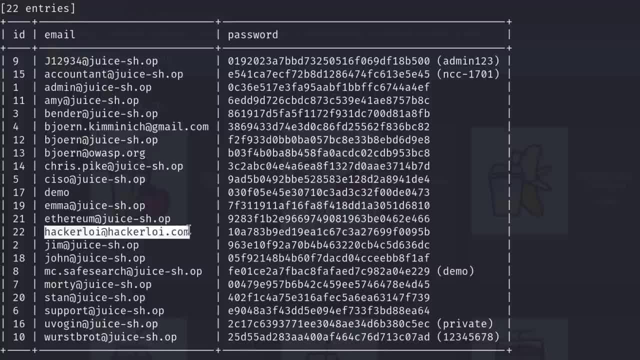 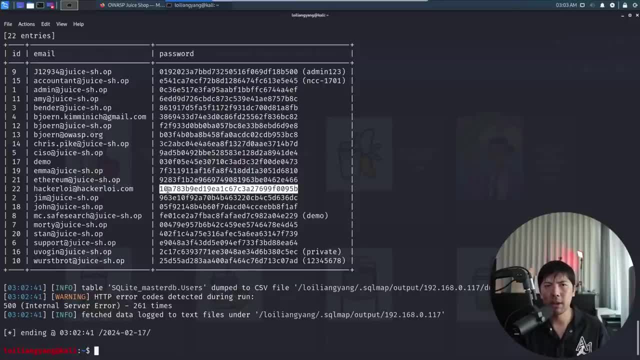 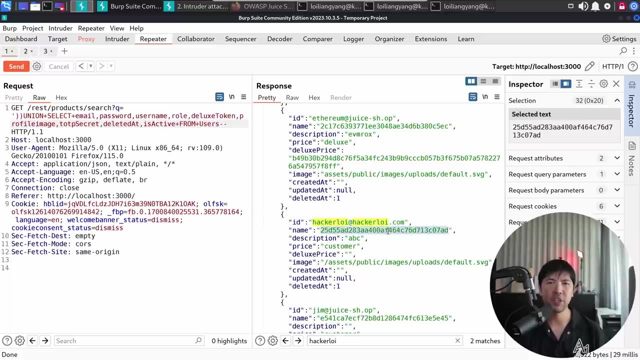 The results here. I know who is Mr Heckerloy. I know him and I know his password. His password is definitely not this, So there may be some kind of mismatch here. So if I go back over into the result from burp suite, you see right here we have Heckerloy and a specific hashed password. 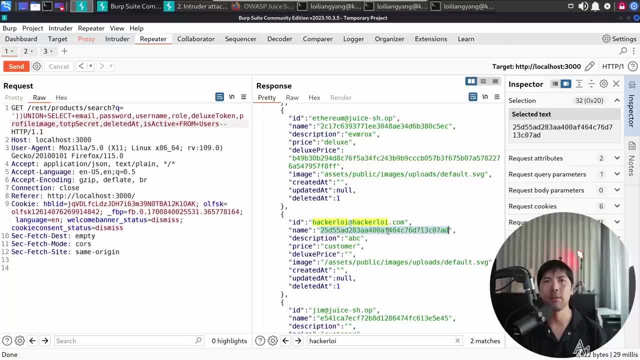 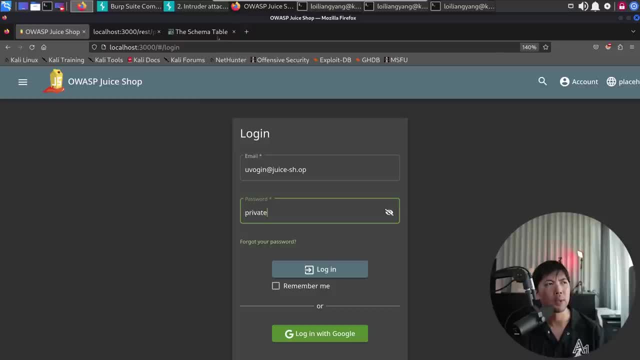 two, five, D, five, five, 80 and so on and so forth. This password is 1,, 2,, 3,, 4,, 5,, 6,, 7,, 8.. So you can easily look that up from crack station. So let's say I go over into crack station. 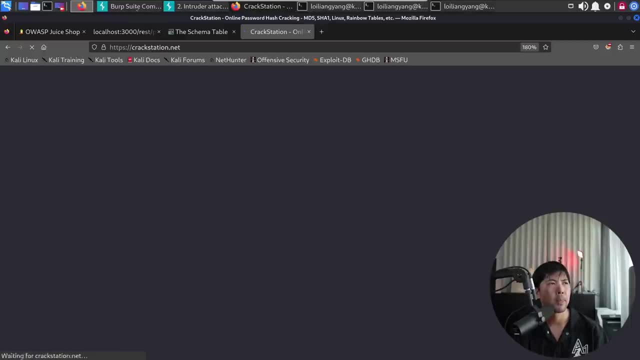 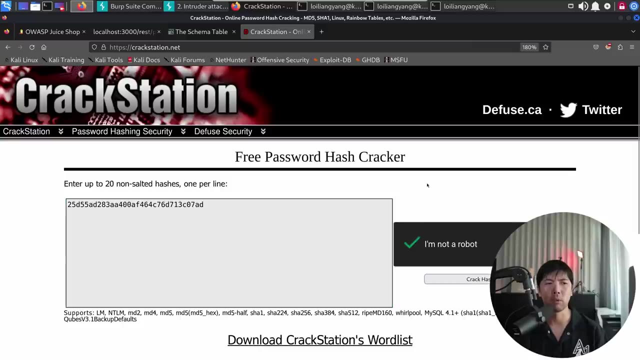 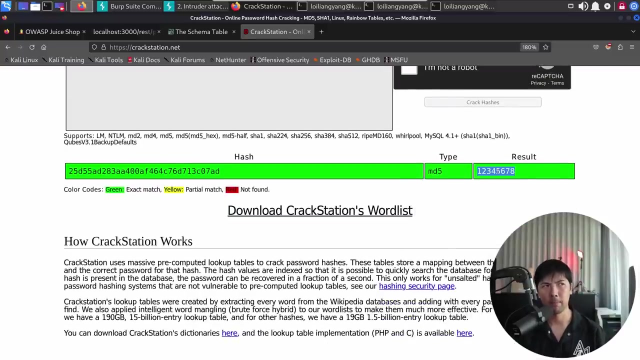 and I look for the online password hash. So in this case can copy the following value: go back to the site, paste it over here. I'm not a robot. click on the crack hashes And we can see right here we have the result of 1, 2,, 3,, 4,, 5, 6, 7, 8.. 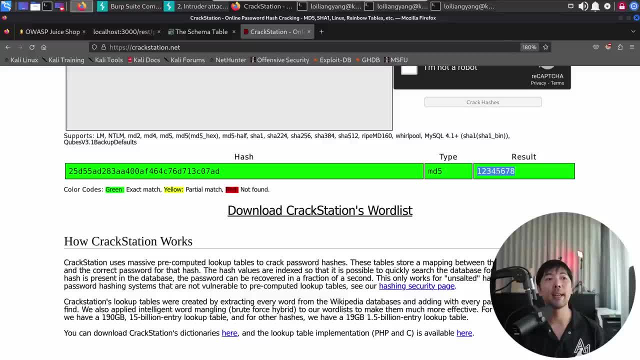 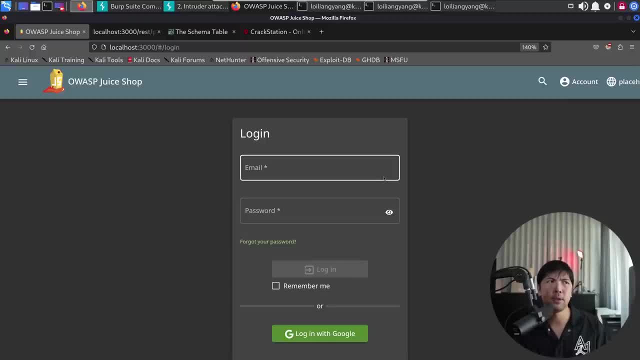 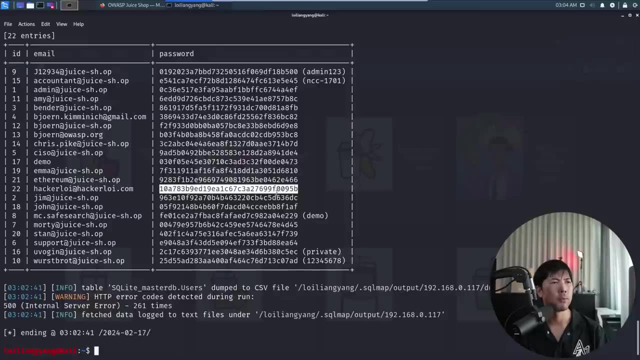 So now we got a password, All right, And we managed to crack some of the values, but we had this match. So what it can do now is I can easily copy and paste those values right here to log into those users. So in this case, if I go over into those corrected passwords, I can see that we have 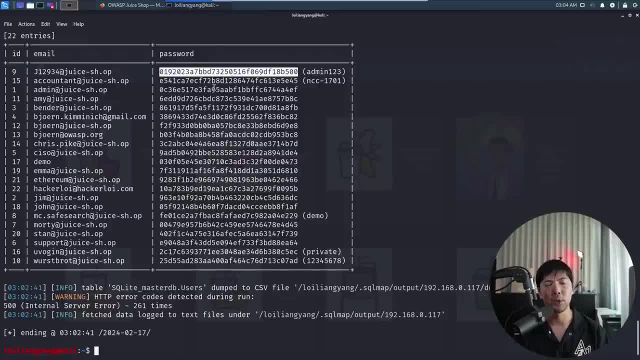 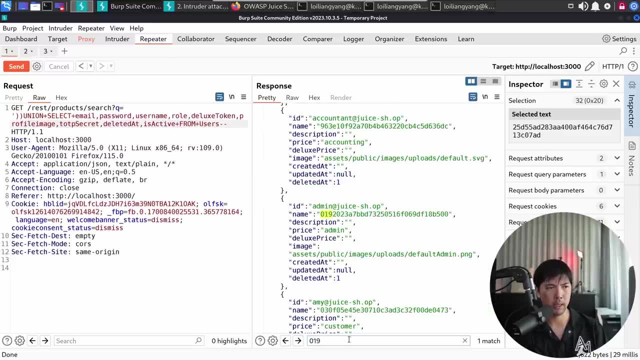 something here which is 0, 1, 9, 2, 0, 2.. So if I hit back over the result here, go back to burp street. All right, 0, 1, 9.. All right, 2, 0, 2, 3.. So this is admin and admin as a password of admin: 1,, 2,, 3.. So 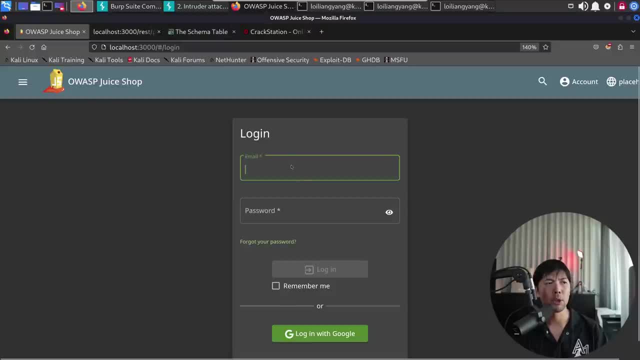 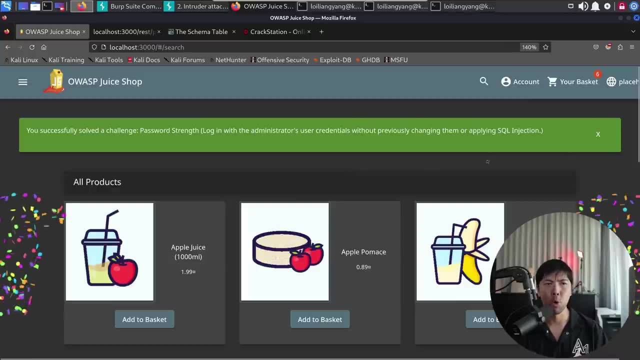 this is the value of the ID, which is the email. I go back to the login page, I paste it over here and I enter the password: admin 1,, 2, 3.. I click on the I show password. click login Boom. 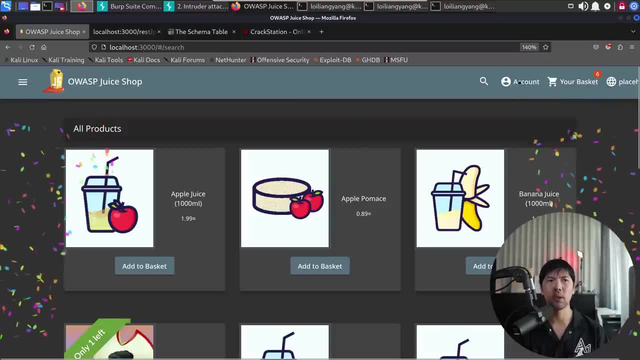 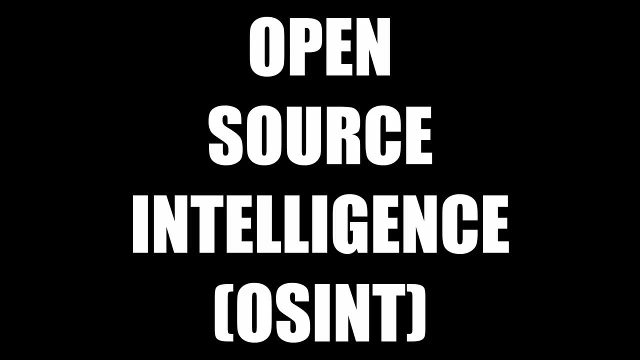 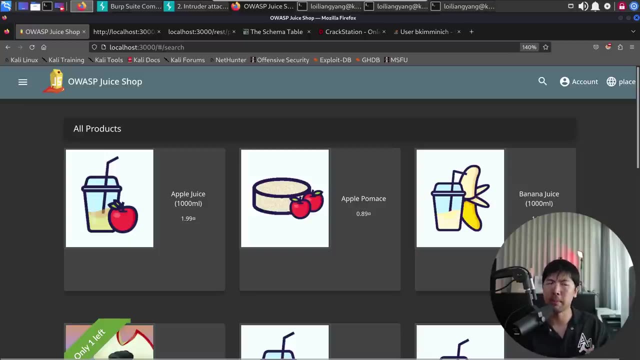 We're in, we've got an access and you can see right here account admin at juice shop. Now the next thing we're doing involves open source intelligence. We are going to be searching about the company, about the organization, the people who administering the company's. 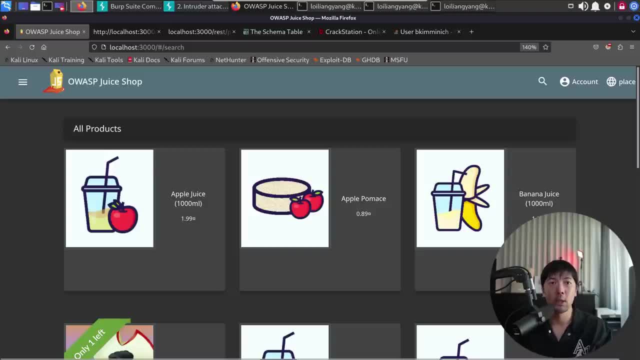 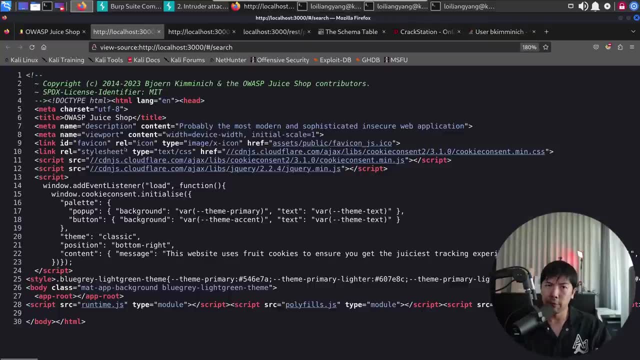 website, because those can give us telltale signs of what's going on behind the scene. So in this case, we're going to do a right click view page source And the first name that comes up is B Kim and itch. All right, So this is someone that we can search for. who is the? 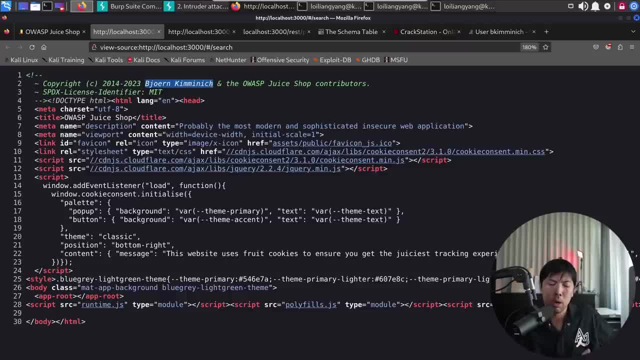 contributor to the site. So in other cases, in a real world organization, it could be an idea administrator to developer and so on And they could be posting questions about, they could be dumping information about the systems for troubleshooting to get help. so those 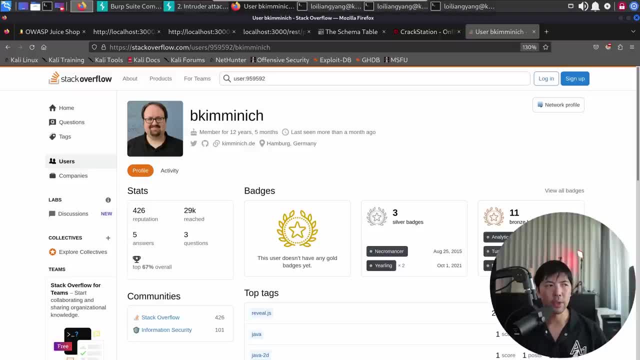 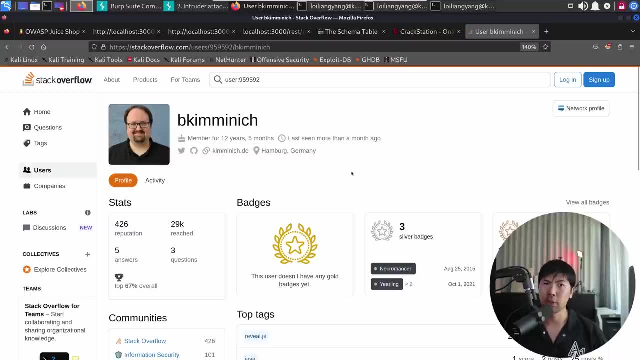 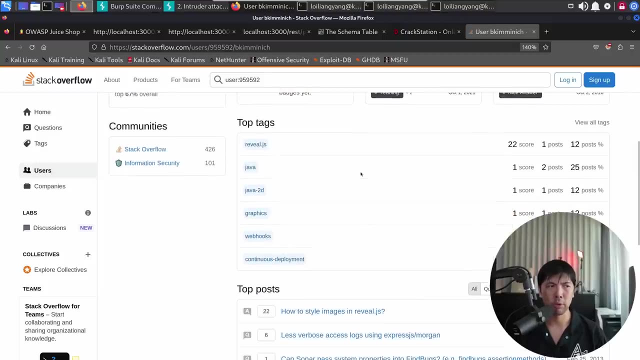 things can happen. so we search for the user and this is the profile of the user. all right, so we can see that kim and itch is based in germany. so we're on stack overflow. this is a place where there are a lot of questions regarding all right it troubleshooting. so if i scroll down further, 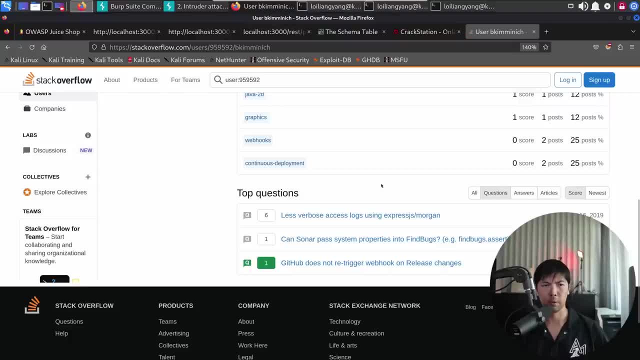 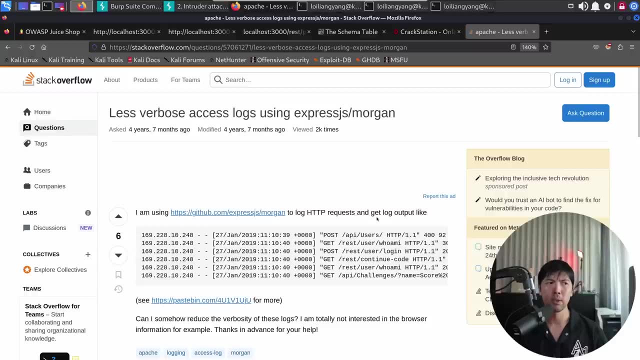 i can say: click on questions and i can see here: all right, there's several questions that have been posted, so go ahead and open them up, because some of these questions could be related to the system that you are crawling through, you're scanning, you're looking for vulnerabilities there. 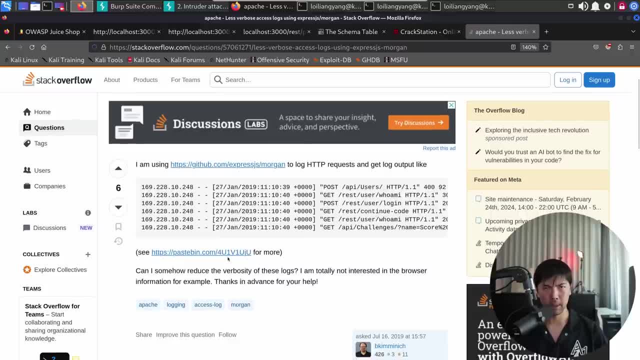 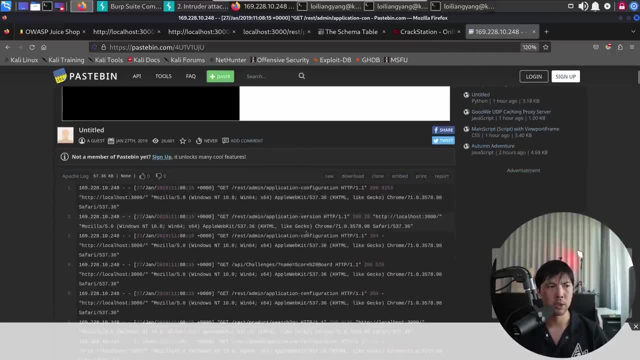 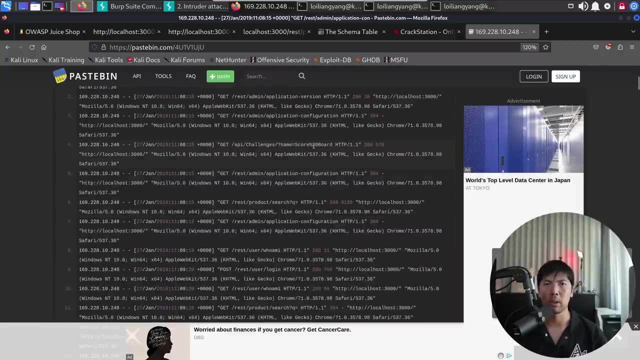 and you can see here, see payspin. so this is a place where you can troll in all this different logging information and see what we get all right. so in this situation we have get rast admin all right. we have all these different details, api challenges and so on. so this gives us a lot of details and we could possibly start thinking. 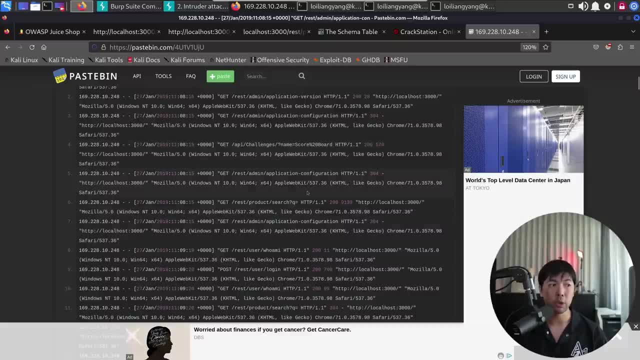 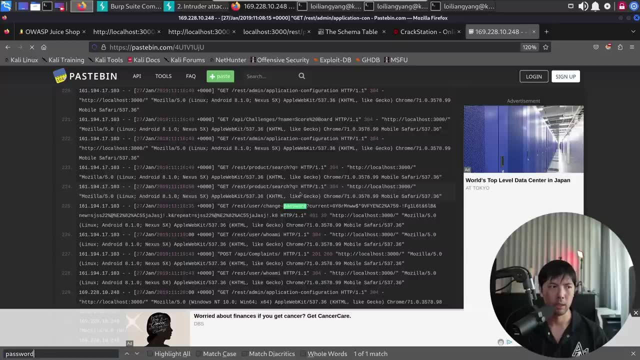 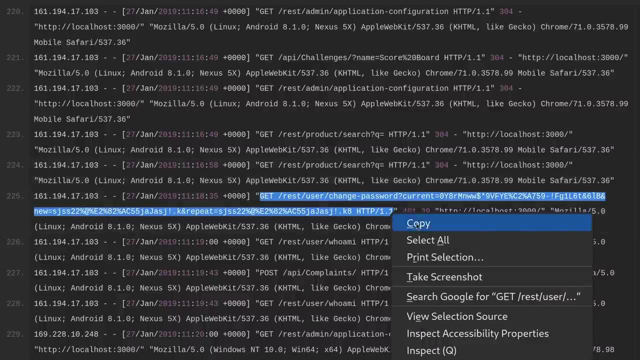 about what if some sensitive uri has been posted here that we can search for. so in this case, if i search for things like password, what do we get? we get something right here. we have the following: i'm going to copy the value out so that we can investigate on this. so let's go ahead and launch. 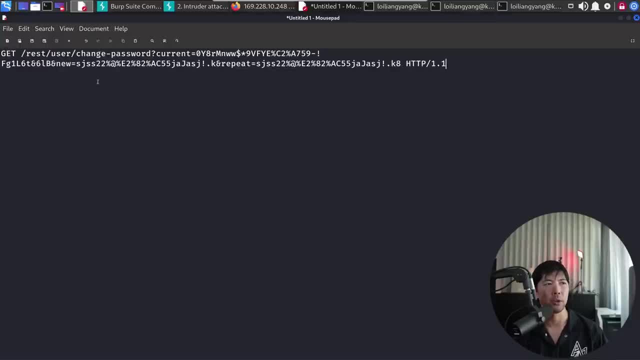 say mousepad, and of course paste it over here. you can see this. change password. remember, when we were doing the password cracking, we did not manage to crack all of those passwords. in fact a large chunk of those passwords were not broken into. so right here there are several values. there is a rest, user change. 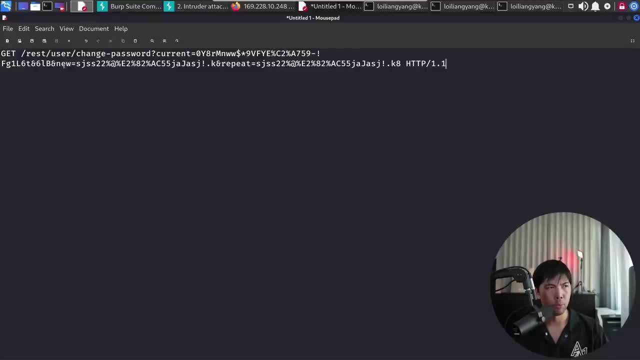 password. there's a current password to supply and then followed by new- all right, and a repeat. so the repeat and the new has to match. so in this case if you see over here new equal and then we end off at n, all right, so we have dot k and repeat equal, dot k8. so perhaps there. 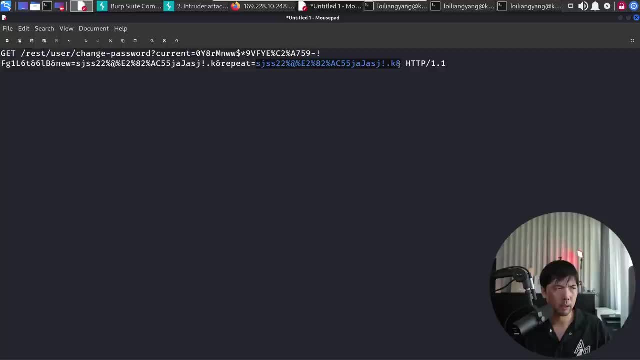 was some programming error so it was not able to work, or or you would just submit it as a log, a full list of log logging events, and it shows up here. so now we have the current password over here and we can try to throw this over into md5. get the value. 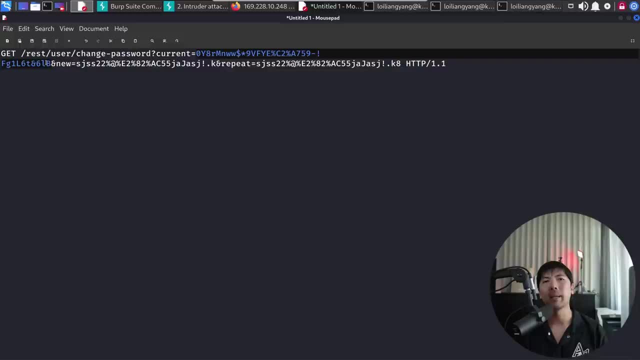 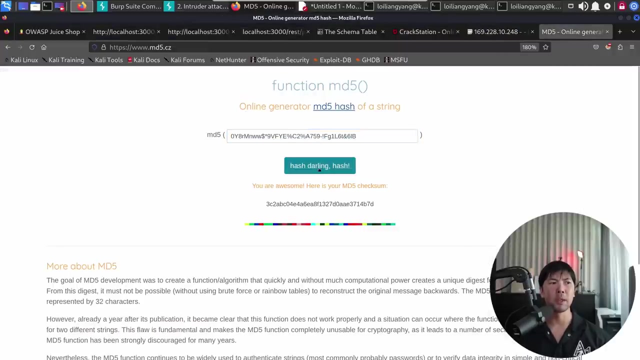 and once we get the value we see which one it matches and then we can log in straight to that user. so now we take the value over here and we throw it into, say, md5. so in this case i have the md5 generator, i paste it over here, i click hash, darling hash and we get the result. 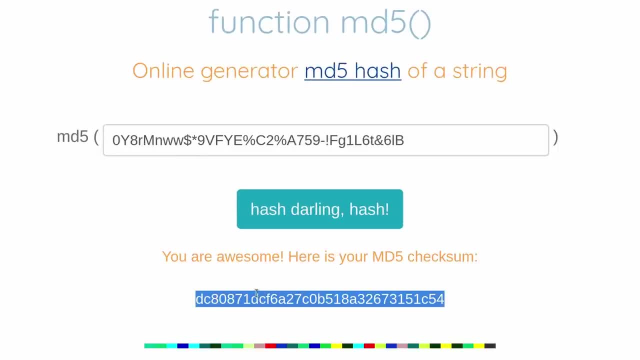 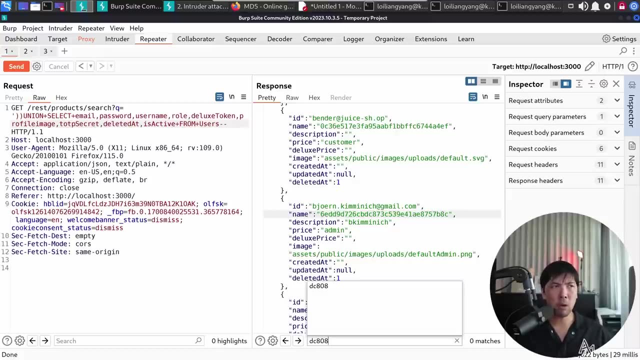 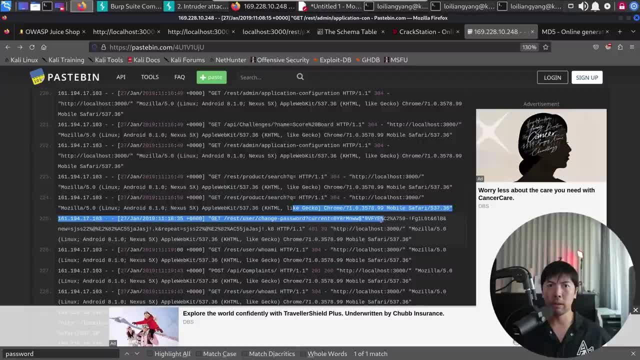 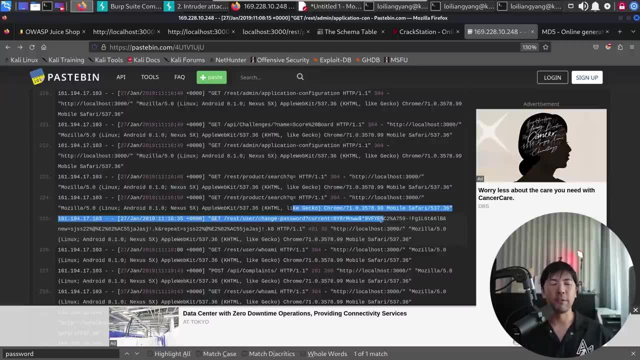 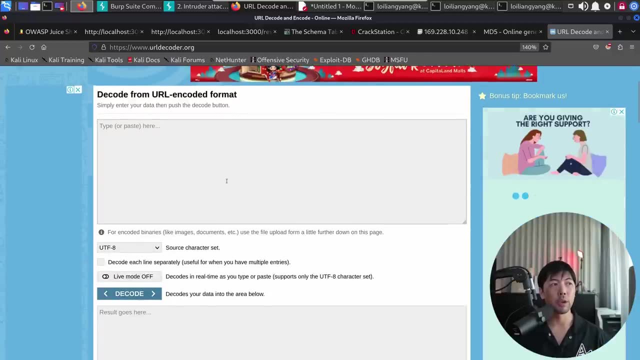 that what we're getting here are url encoded, meaning that the payload or the value we've gotten has to be decoded first before we throw it in to the md5 hash. so you can see, here i'm going to url decoder, i'll paste the value here, click on to decode and once you get the decoded, 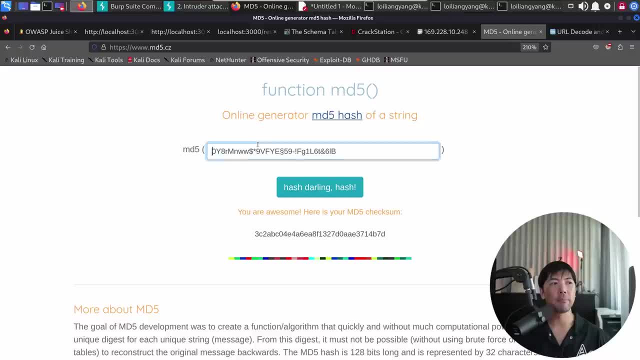 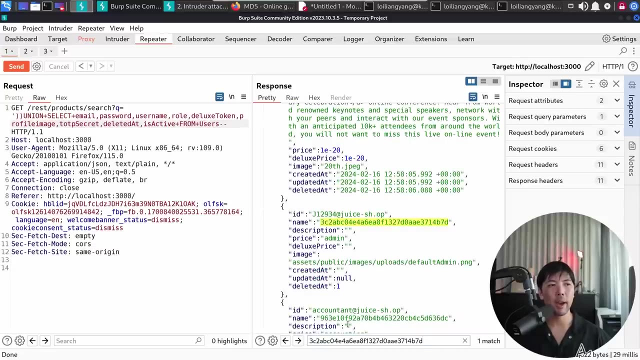 value: copy it, go back to md5, paste it over here and click hash, darling hash. so right now we have the following value: copy this value. i'll go back over to burp suite. i'll go over into repeater tab. i'll paste the value right now and we get the following: 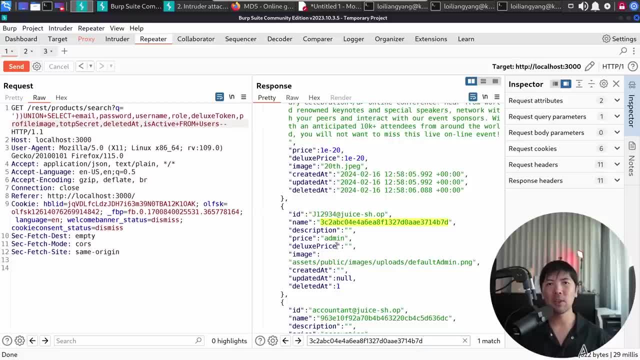 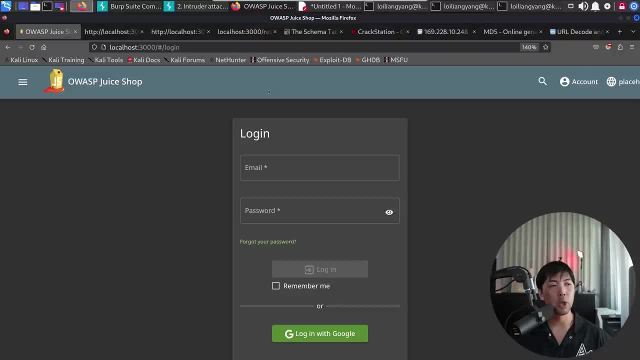 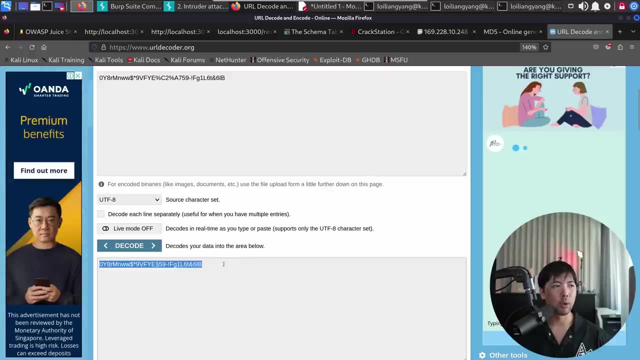 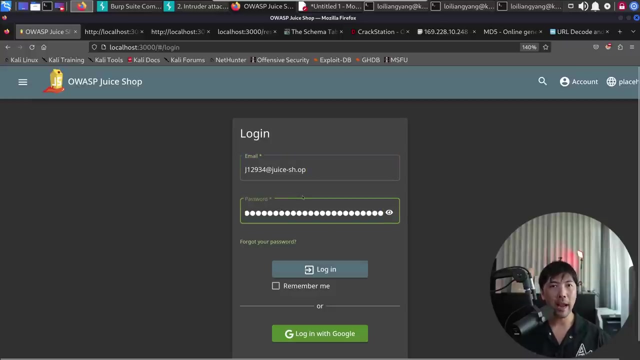 j. one, two, nine, three, four has this password. so what i can do now is can copy the id: right click copy. go into the website login page and get that password, the password that we have decoded over here. do a right click copy. go back over into the login page. paste that password. 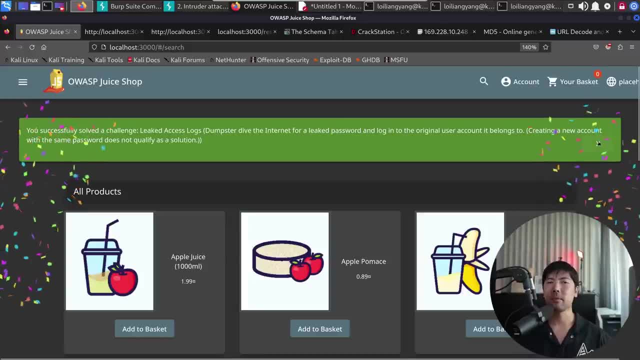 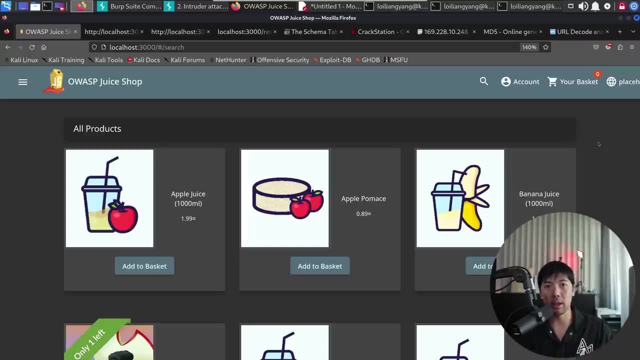 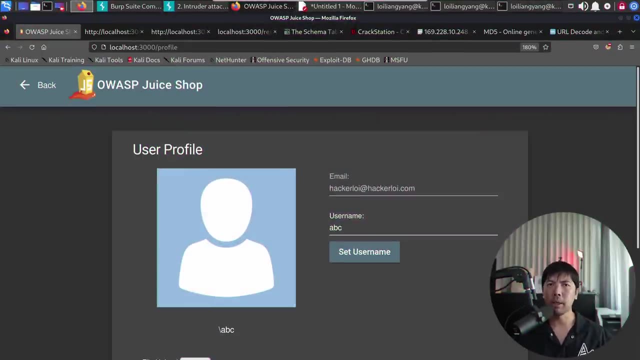 click login. boom. we have used information through open source intelligence to get us access into the user's account. moving on, we are also looking at entry points that allow us to do some kind of data entry that could possibly lead to some kind of command injection. so in this case, if you 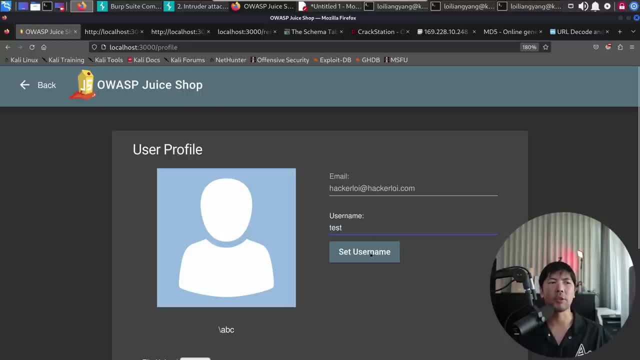 see over here of username. I can enter abc, I can enter tasks and it reflects back onto user profile. and the first thing you may be thinking of could be cross-site scripting attack. and you are right. it could also be operating system command injection, where we could send some kind of remote command injection over into the profile or into 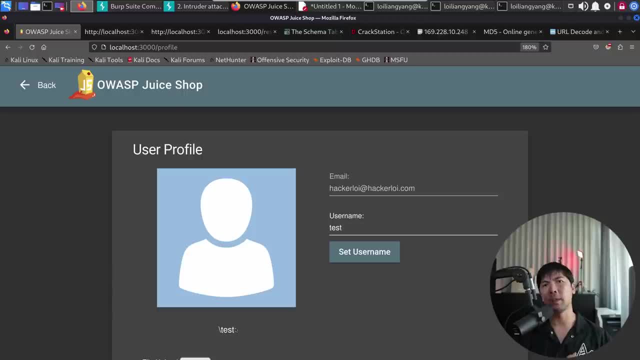 the entry point and then after that, gaining control of the entire site, and that's the aim we're going for. so if you see over here a specific payload that looks for a calculation of one plus one, and I click set username and we get a result of two, so why is this happening? so I have a specific payload. 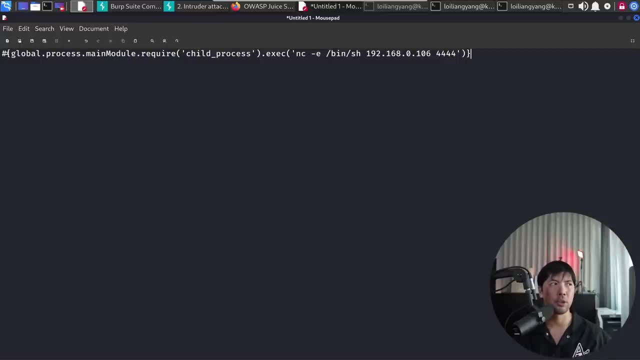 right here that give us access to the entire server. once you upload this code with netcat-e bin shell to a target address, which is the hacker's address that's listening, it gives us remote control of the entire website. here I have another colonics that's running and we're starting up the listener, so I hit enter on. 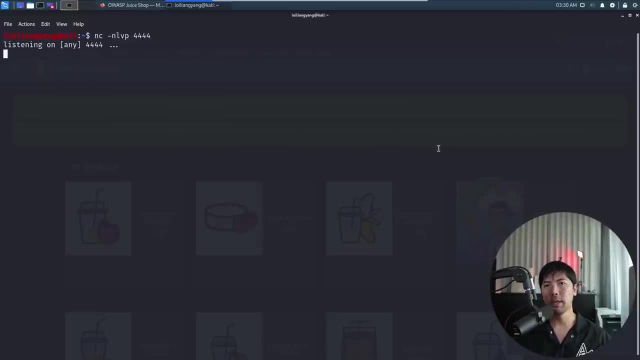 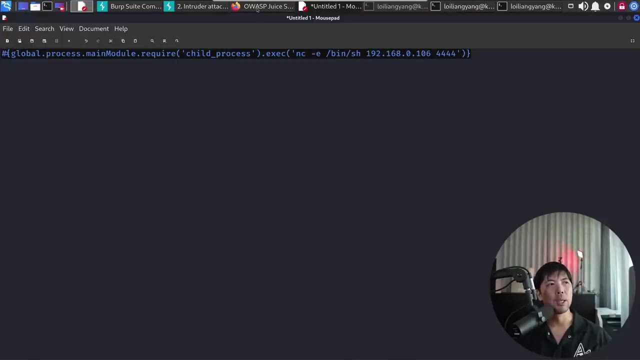 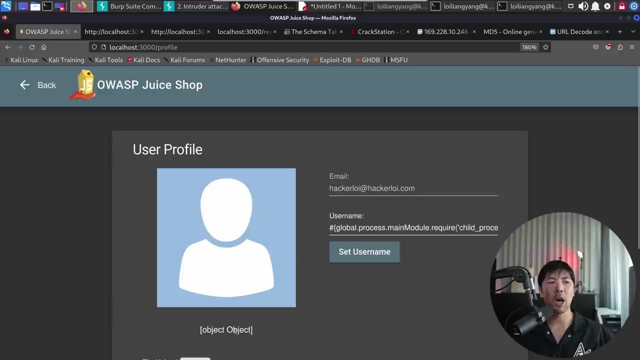 that we're now listening. and if I head back over into the target server and we can load command over into the entry point, I copy this. I go back over into the profile. I paste it right here. I click set username. we can see object, object. I head back over to the other colonics that I have. 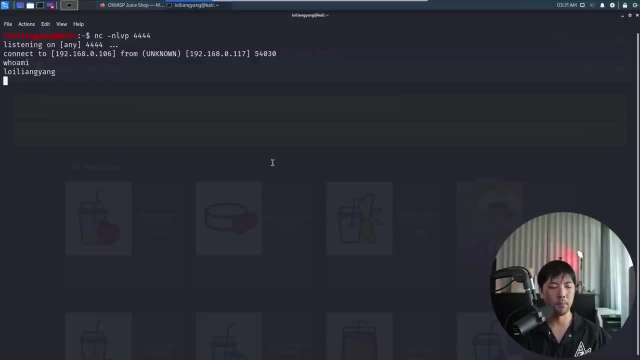 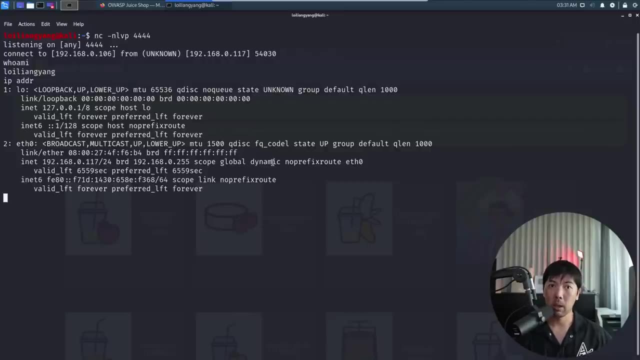 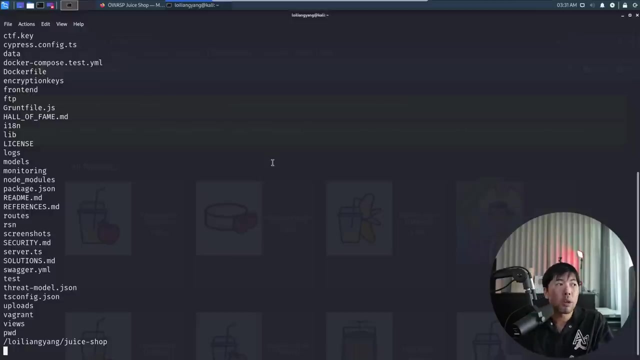 I can now enter who am I and boom, we are in. we now have access and remote control of the entire website. I can enter, say, LS, I can see my print working directly. I'm able to now navigate across the entire site, giving us full remote control of the. 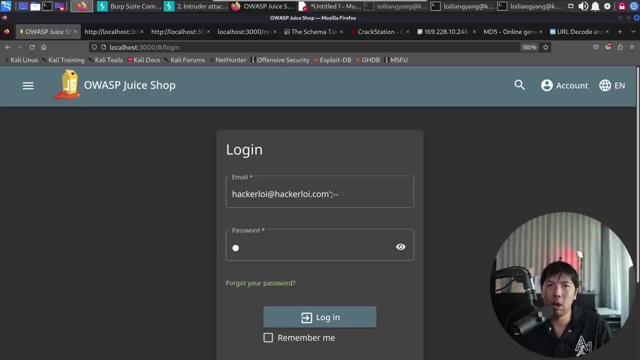 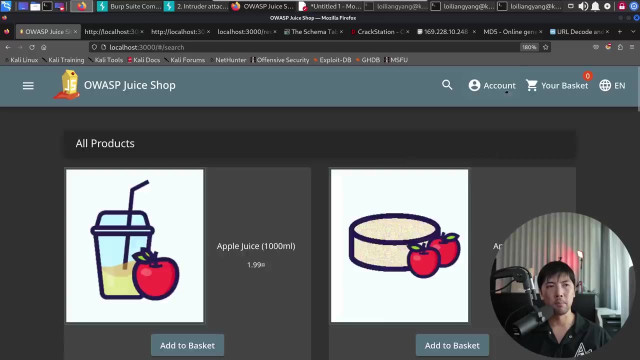 website if there is a vulnerability directly in the login field. you don't even need to know any of this attack methods. all you need to do is to have a sequel injection entry right here with a single quotes: semicolon, dash, dash, click login and boom, top right corner. you have now logged. into the user. you don't even need to know the password and pretty much click and running. we will 들�降 in. you will now log in to the user. you don't even need to know the password. so if I was a chat, you don't even need to know the password. so if I was a chat, 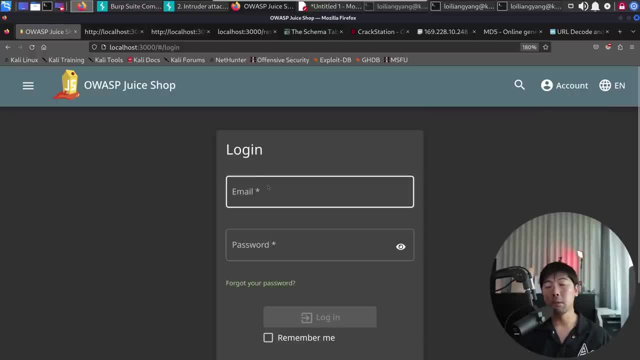 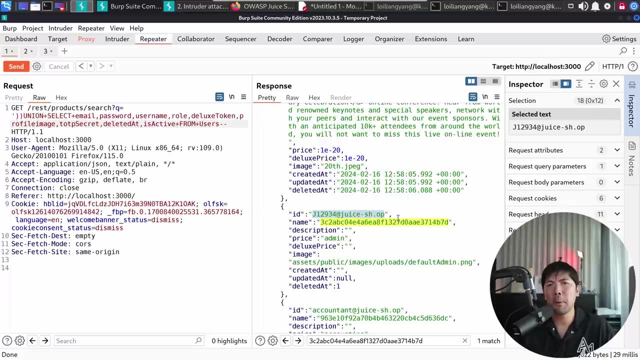 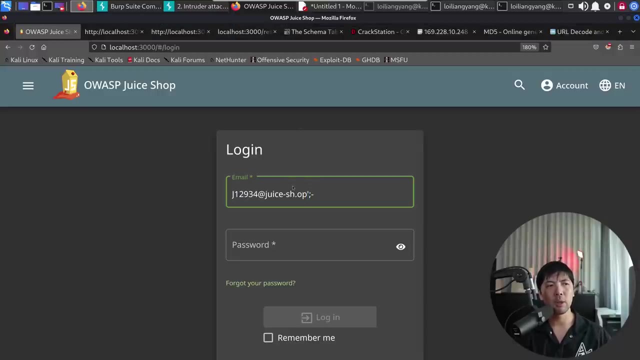 try it for the earlier user that we were enumerating, say, for example, i go back over to burp suite and i want to target this user and we went through so much pain to get the user's password. but right now, if i was to paste the value over here, single quote, semicolon, dash, dash, because 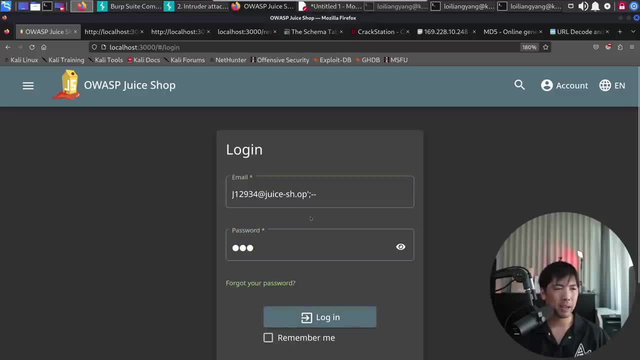 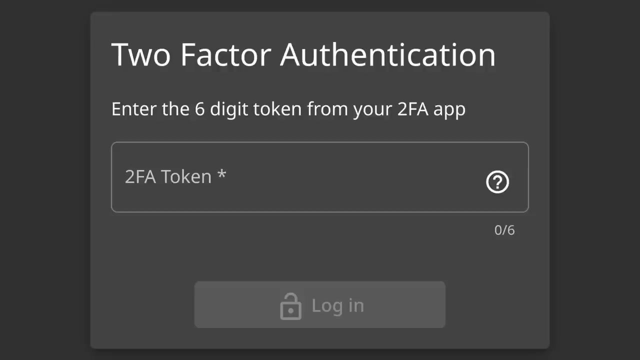 of the vulnerability. i enter whatever as a password. okay, i click login. boom, top right corner. we are in once again. however, you may get into a situation like this: you click login and it prompt you for two-factor authentication. you're stuck now. what can you do? what you can do now is go back. 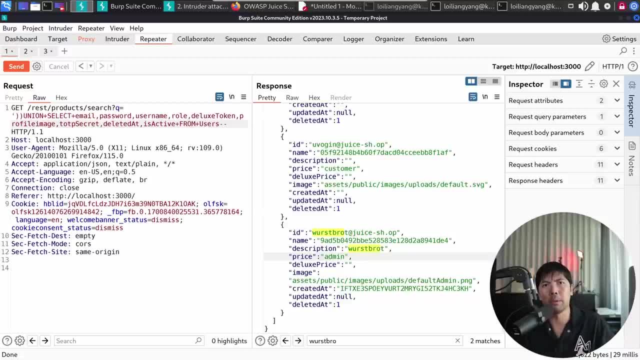 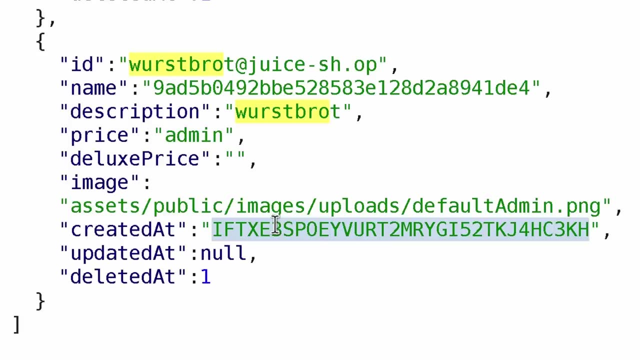 to the earlier result from sql injection, which allowed you to dump out all this information, and there's one specific column here called totp secret, which stands for a time-based, one-time password, and in this case we have a specific value here and this value is allowing us. it gives us the ability to connect to something. 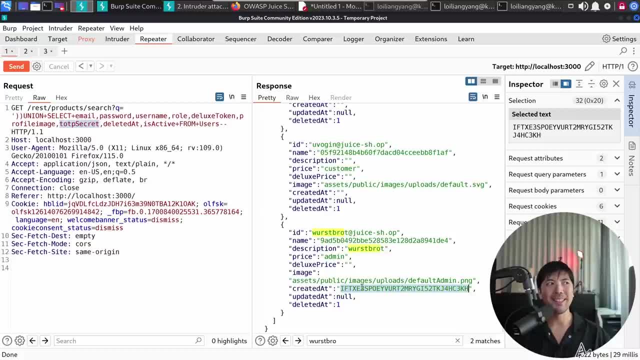 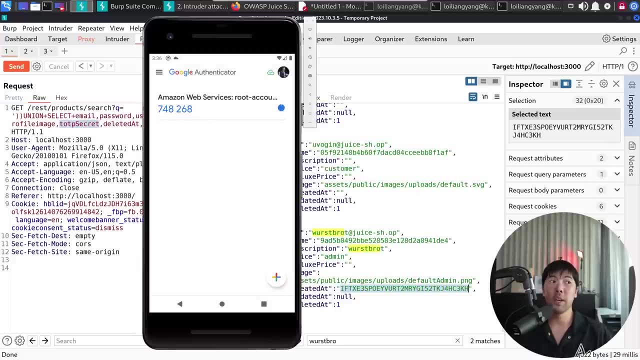 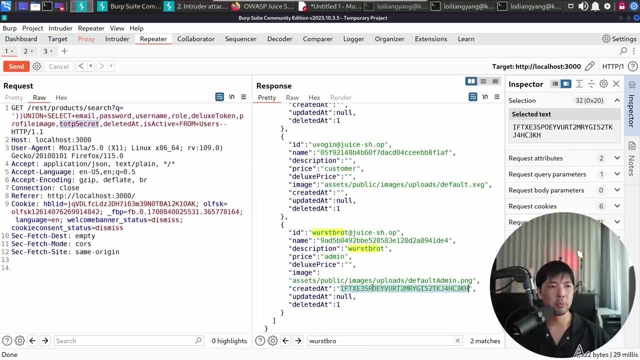 like an authenticator. you input this value and then it generates the time-based, one-time password for you that then allow you to log right in. so in this case, i have my google authenticator running right here. i'm going to do a copy of this value. all right, right click copy. i go back over to my 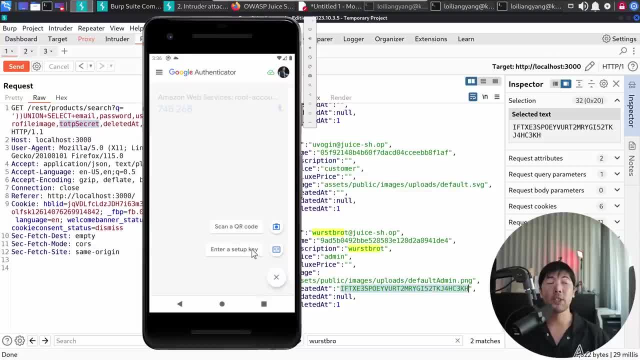 mobile device, i click plus and i enter a setup key. all right, i call this, say hacker loi and i paste the key right here. okay, let's go ahead and copy this one more time, go back to my mobile device and see whether i can paste the value here. if not, i'll go ahead and 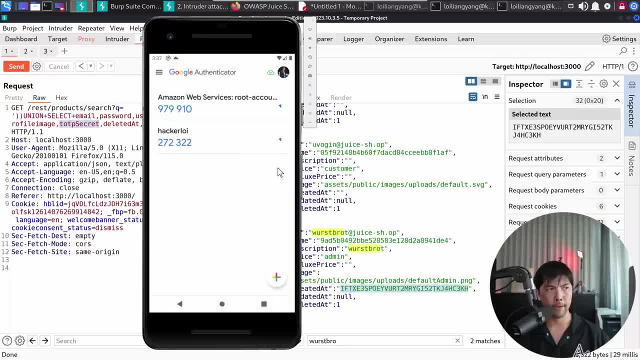 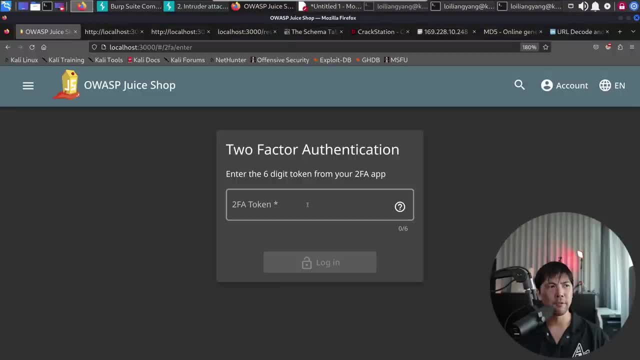 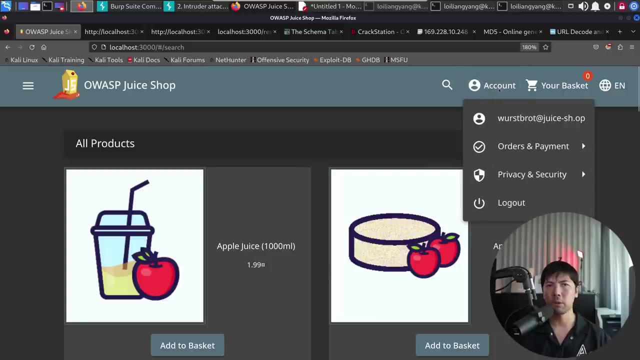 enter it. i've entered the key. right now i click on to add and we can see we're constantly loading the time-based one-time password. i go back to the login field. here we have the two-factor authentication. let's go and enter the value here: 079101, 079101. click login. boom, see the top right corner, and we managed to bypass the.